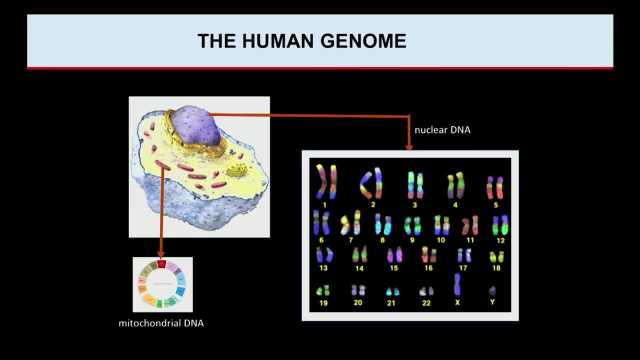 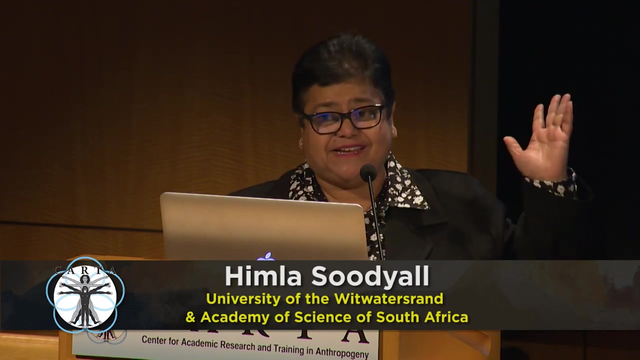 which is DNA, And we have two types of DNA that carries the blueprint that we all walk with- And I know to this audience this is like kindergarten school, But I'm showing this to remind us that I'm going to talk about two different types of inheritance: The nuclear 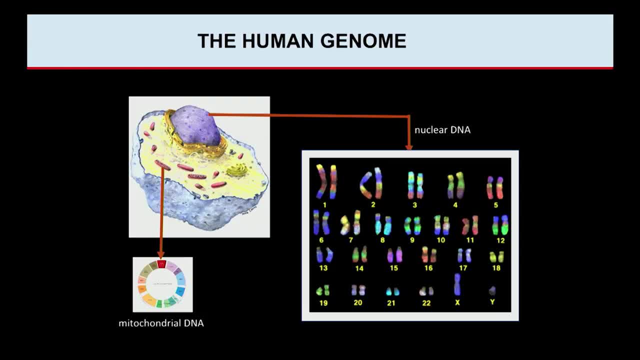 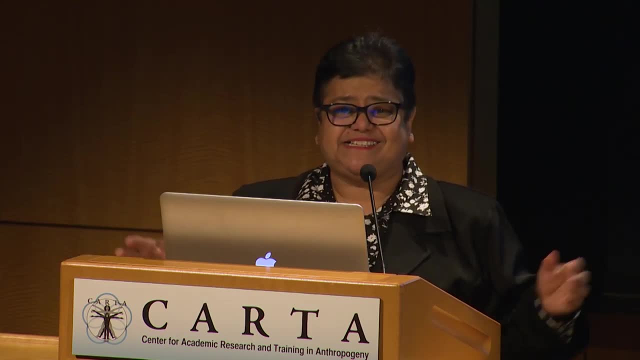 DNA, which makes up the chromosomes that undergoes mixing at cell division or recombination. That is now why I am at this height and at this size. You heard about brain size and height and weight, etc. Well, I am your show and tell. 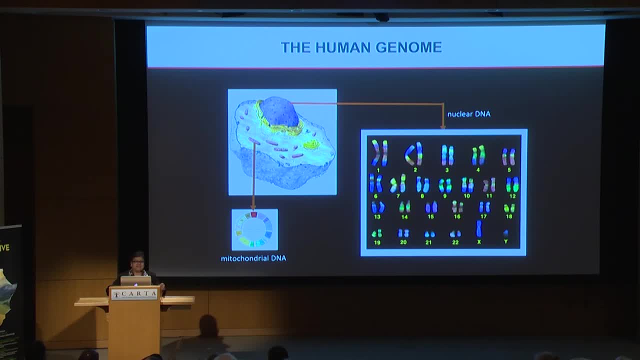 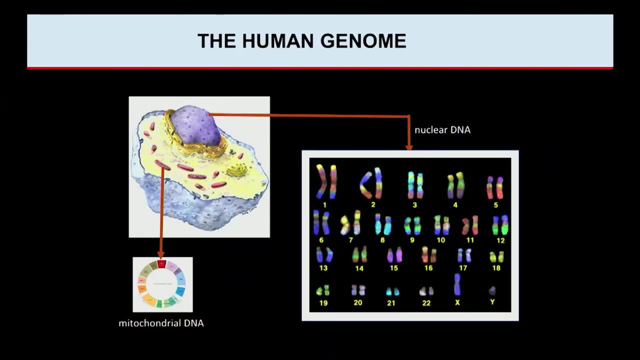 for all of that today. In addition, small is packaged and dangerous. We have the mitochondrion that has its own unique set of DNA which, over evolution, has come to carry yet another remnant of DNA in every cell. Now, the reason why the mitochondrial DNA is of use is that 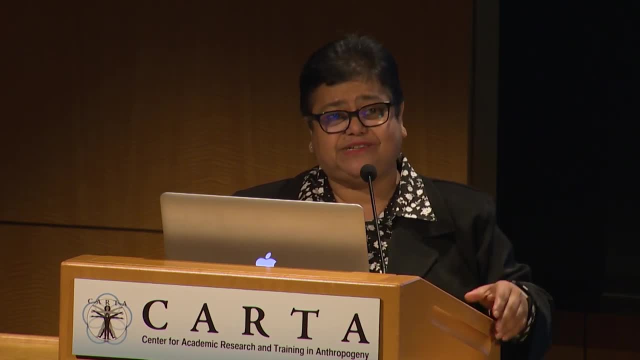 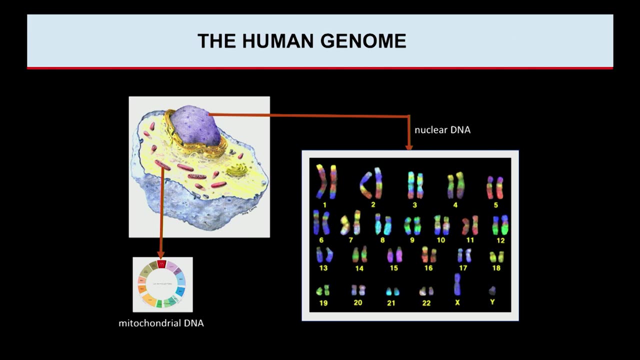 it is genetically, maternally inherited and carries a trajectory of our maternal inheritance. So these are my two show and tell sources of information, And so that I don't exclude the males in the audience, Yes, you have that little thing there, The Y chromosome. Well, 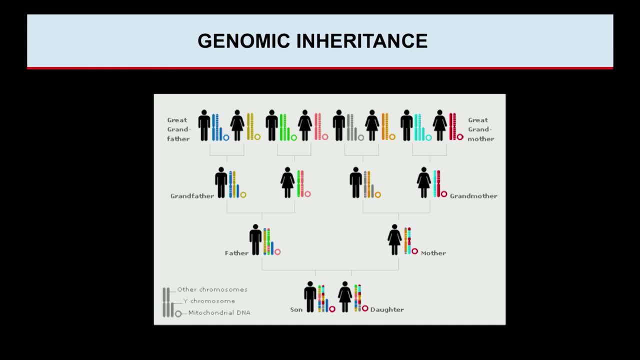 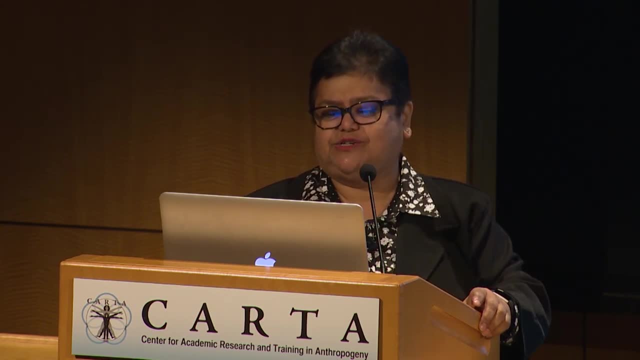 genomic inheritance is known to all of us. We get half our chromosomes from each of our parents, And they are from their parents before, and so on and so on, And so, with respect to mitochondrial DNA, we would be able to track what both sons and daughters got from mother, from maternal 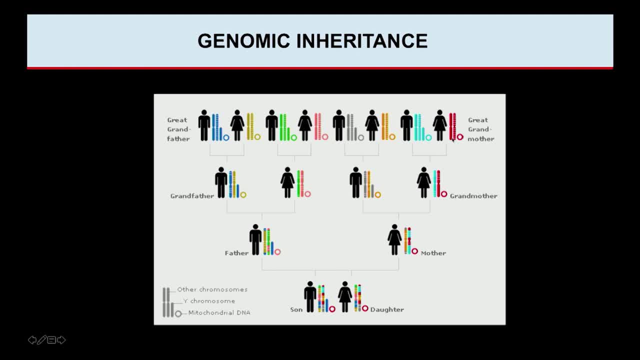 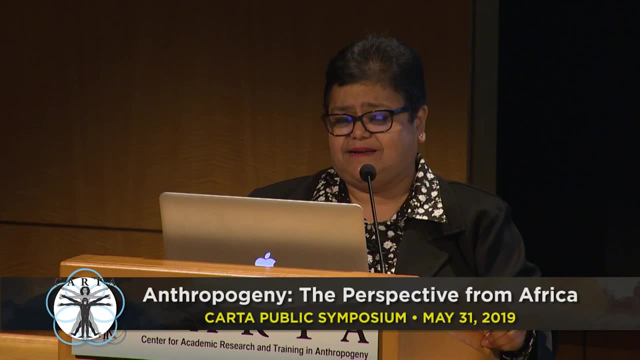 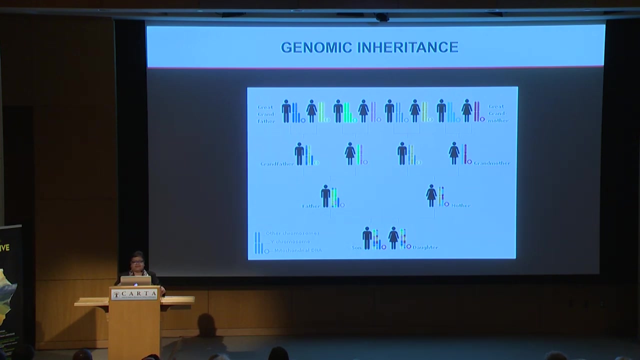 grandmother and great grandmother and so on and so on and so on. In males who have the Y chromosome we have the equivalent mechanism to trace paternal heritage, But of course The nuclear DNA carries the contributions from both parental sides And if you go back one, two, three generations, you have eight people who potentially contribute to your ancestry. 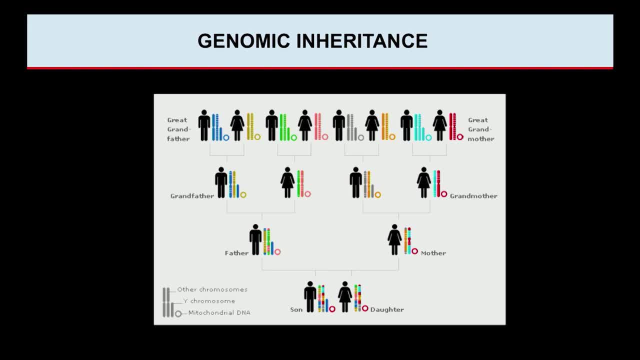 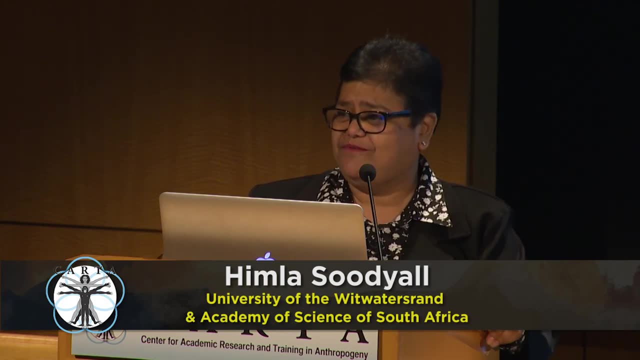 And if you want to go back 20 generations, two to the power. 20 would have contributed to your total genomic information, But you'll still have a single maternal ancestor, And it was just by chance that I chose for my title. So Where Do We Come From? 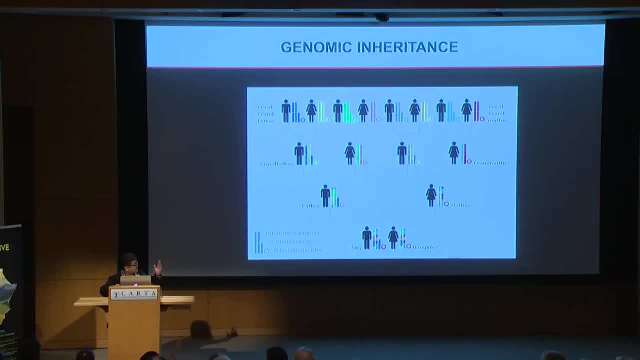 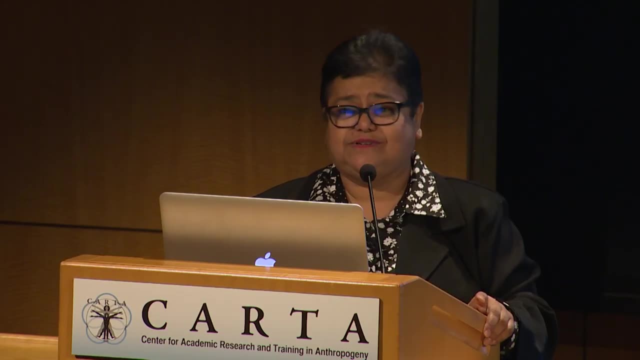 Not knowing that. that is among the questions that Carter looks at And the reason I chose. that was about 15 years ago. I was involved in a documentary that was produced in South Africa by one of the TV networks by the same name And in that we showed peace. 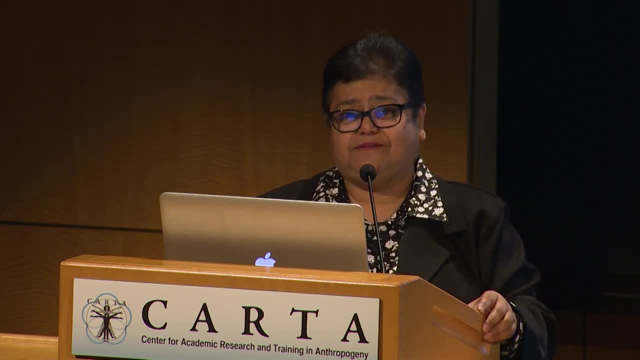 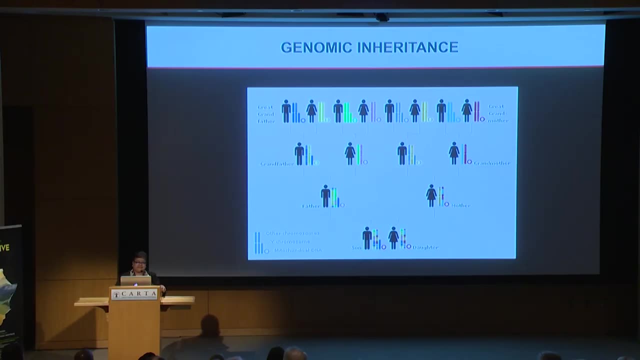 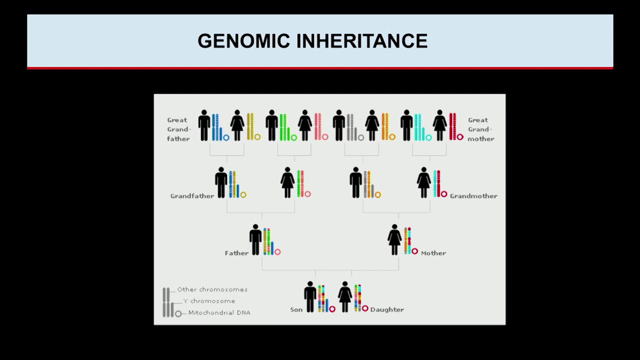 A whole bunch of local people transcending politics, sports and all sorts of disciplines, And we did their genetic ancestry tests and made a story out of it And I was going to show you some clips from that but it would have eaten into my limited time that I had. 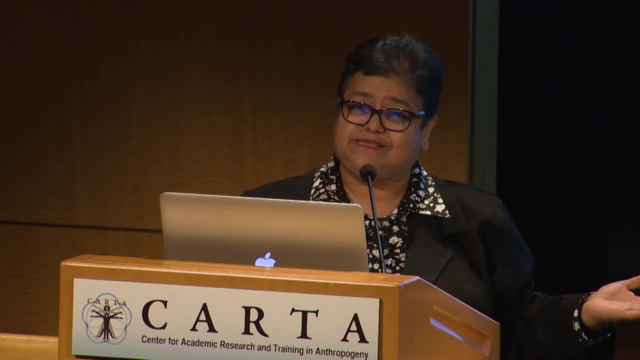 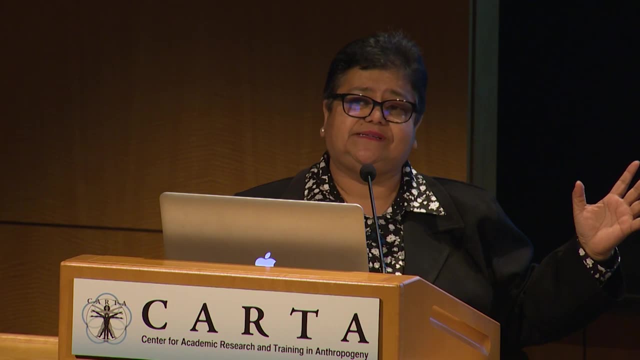 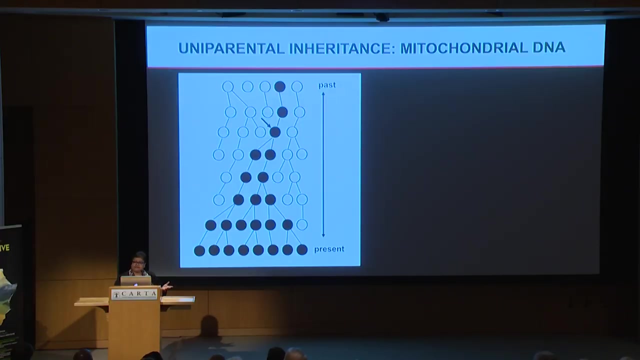 But in any event, you've heard about fossils, You've heard about tools, You've seen a little bit about culture And basically, Basically, those sub-disciplines allow us to track from the past and build up to the present. The genetic toolkit is the reverse. 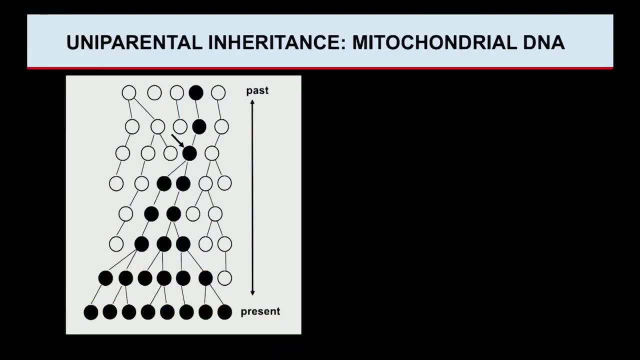 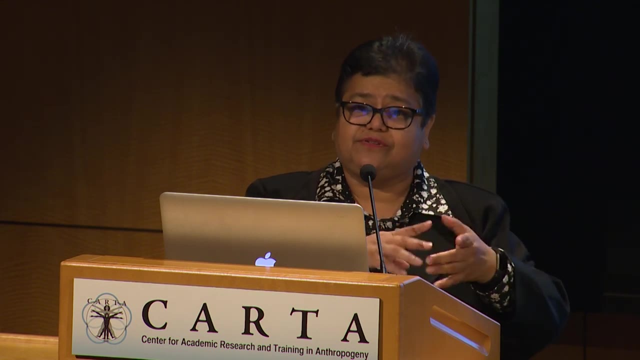 We study the DNA found in living people and we reconstruct the changes over time. And for this demonstration I'm using mitochondrial DNA which is only transmitted through the mother line to daughters and only daughters will pass it on. And the sexy thing about this DNA is that it does not shuffle or recombine. 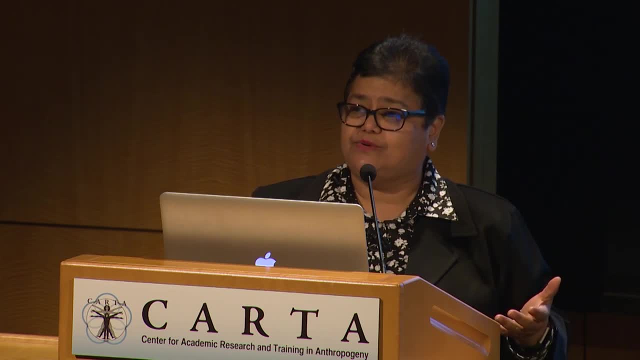 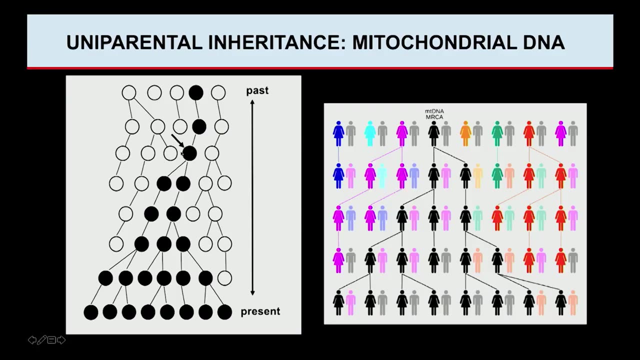 So you have a mechanism and a valuable tool to reconstruct the history of change over time to some point back in the past. And if I were to demonstrate this with a little bit more of a cartoon? so if we were to take mitochondrial DNA, we'd be able to link it to some point back in the past. 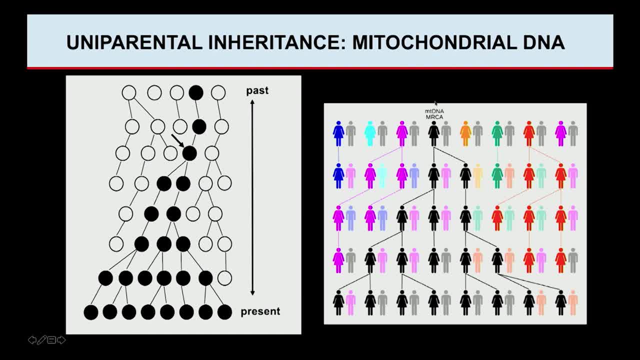 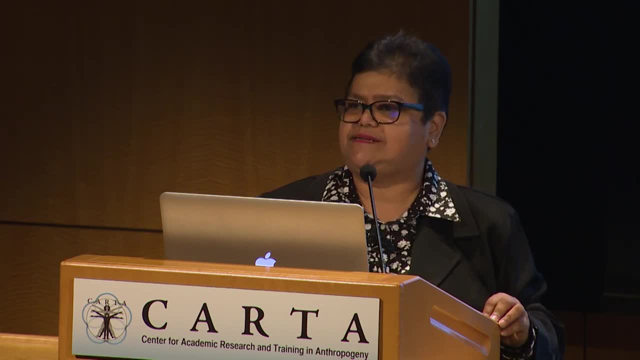 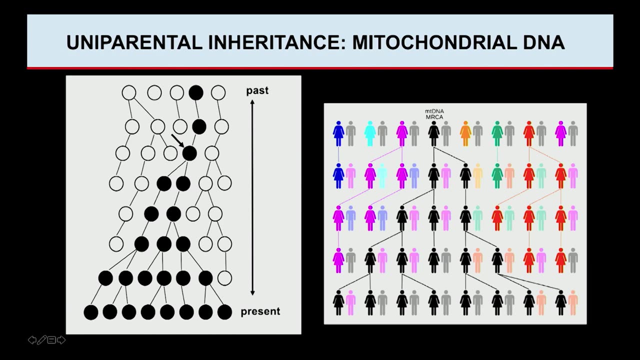 We call that the most recent common ancestor, And the reason why I dislike the use of the terminology mitochondrial Eve. it gives a sense that the most recent common ancestor was the only female present in that time zone, which is not the case. So, but in reconstructing the lineages found in living people, the divergent lines kind of coalesce or come together at a common point. 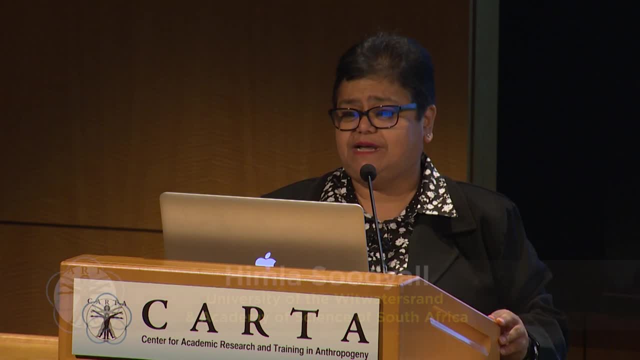 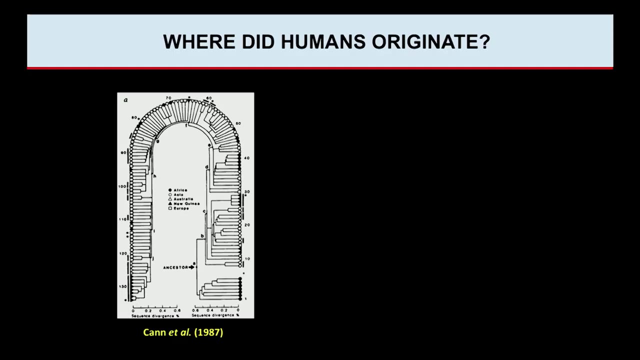 Some In the distance past dated to between 150 and 200 thousand years ago Now. mitochondrial DNA was made famous by the seminal paper by Becky Kahn, Mark Stoneking and Alan Wilson, where they used mitochondrial DNA, And in the 80s we didn't have the sophisticated technology of polymerase chain reaction to make lots of copies of DNA from small amounts. 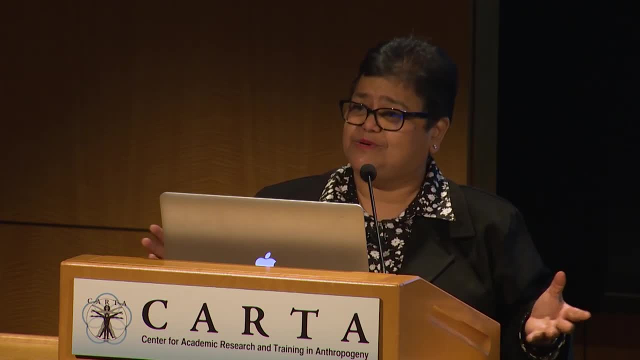 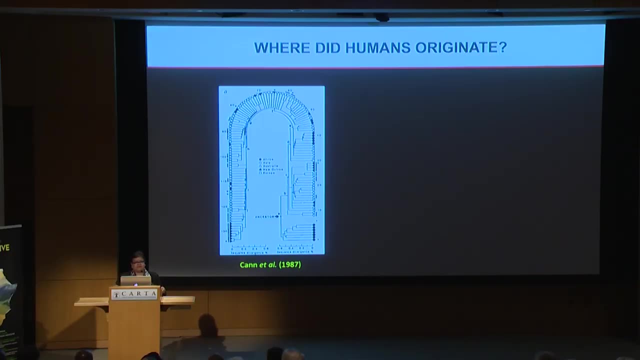 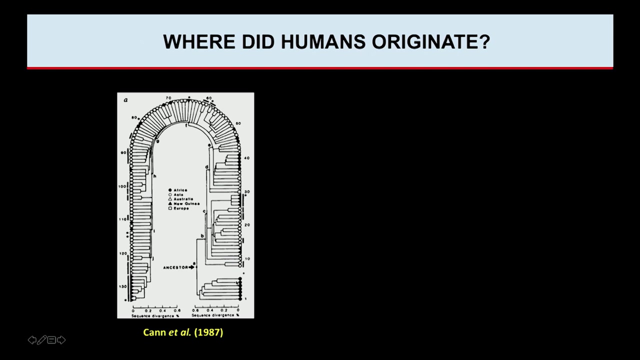 These authors went out, collected placenta, which was a rich source of DNA, extracted the DNA, cut it up with little protein tools called restriction enzymes, and created these maps. And what they found was, when they looked at the relationships of all the different patterns that made up the lineages, one particular branch was exclusively containing individuals from Africa. 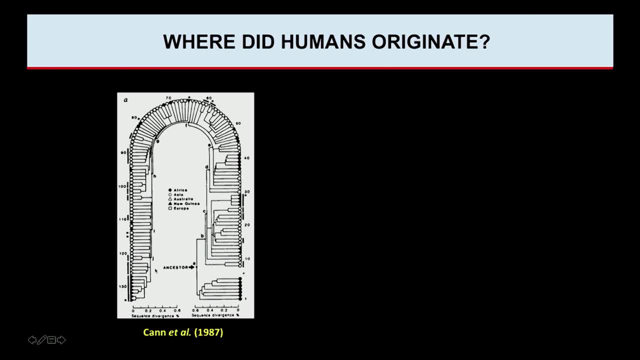 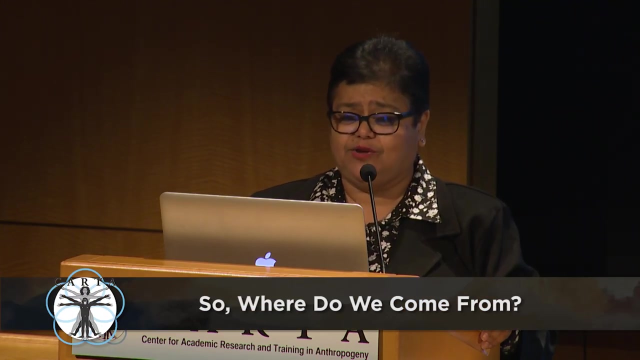 And as you went towards the rest of the tree, drawn here as the famous horseshoe-shaped tree, one found that in the shallower parts of the tree, individuals from Europe and Asia were positioned. So this kind of steer-headed or the out-of-Africa theory concerning modern human origins, it wasn't without controversy. 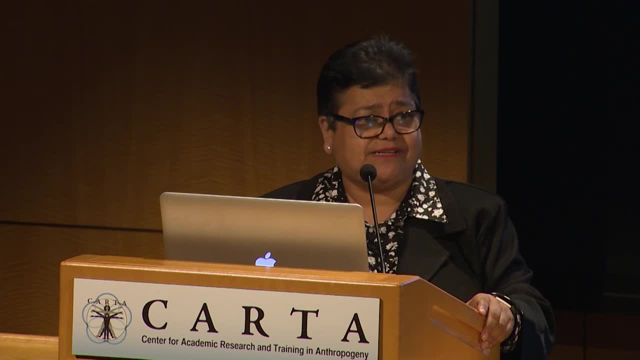 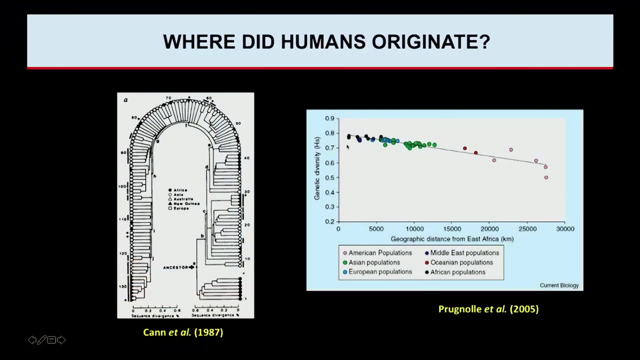 There were many, many scientists. There were many side chirps around this criticizing the technique for the dating methodology and so on, But that's a long story. But several other types of studies started to come to the fore And what was now becoming more and more apparent was that, as you went further away from Africa and for our colleagues from East Africa, that's seen as the center of the evolution of our species. 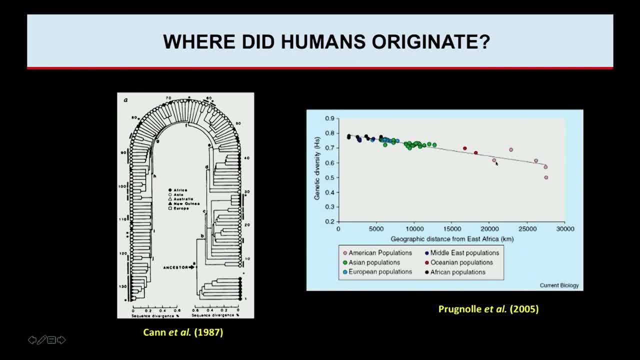 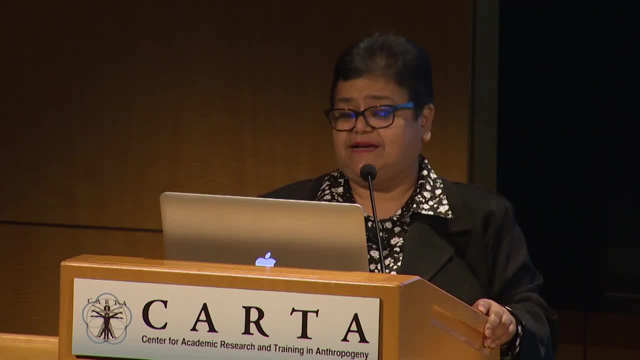 as you went further away from Africa, the amount of genetic diversity was becoming more and more reduced, And this was further evidence that our species originated in Africa. I don't think the world was still ready for this, because, I mean, just think about it, you know all the social issues going on about coming from Africa, and that's like another five lectures to go, but I will spare you that. 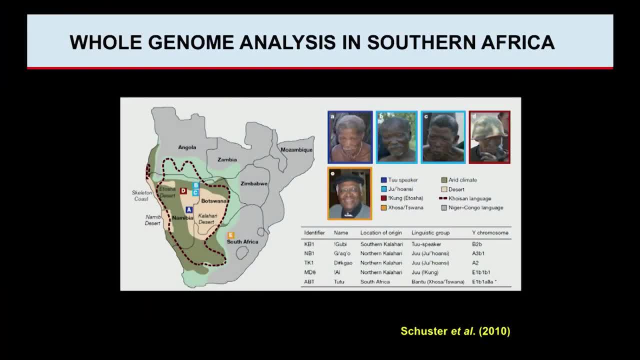 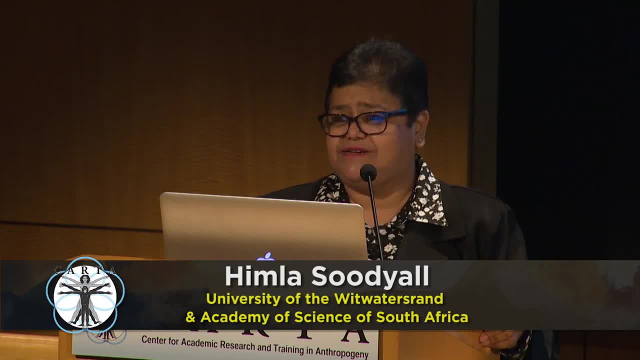 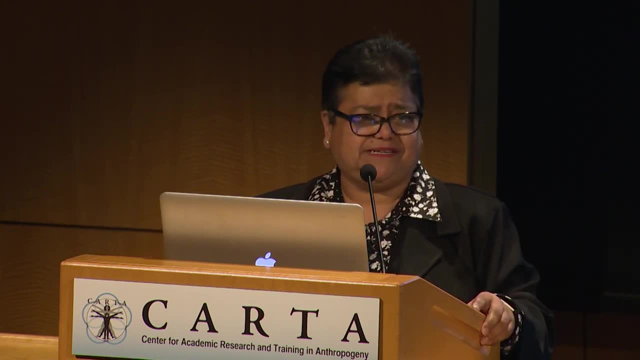 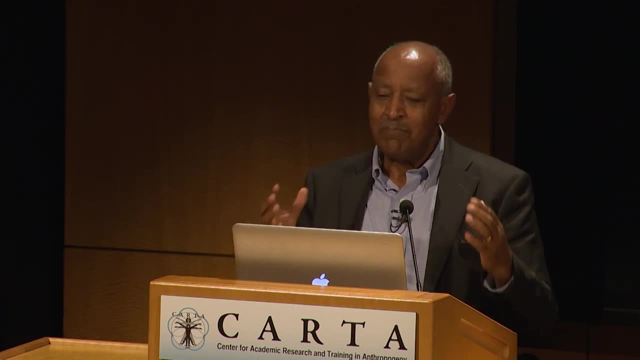 The culmination of the Human Genome Project gave us scientists, you know, an open era of asking questions and trying to resolve that through research of morphology or features. but for the purpose of my talk I want to limit it just to the face and small regions. 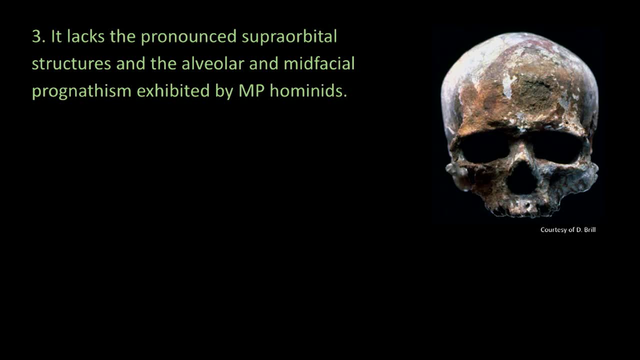 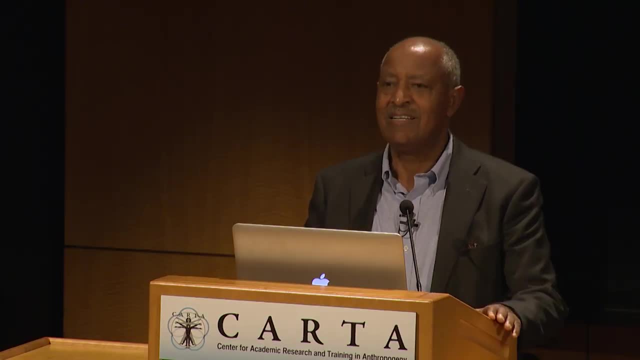 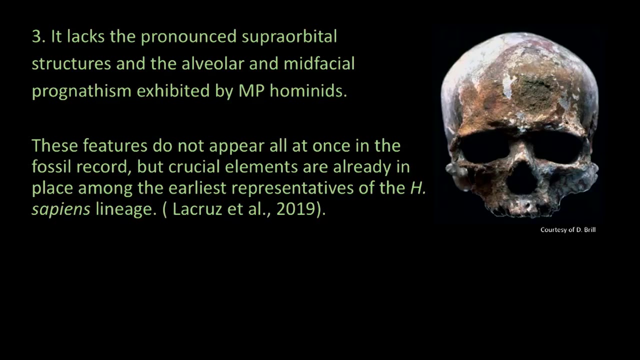 It lacks a pronounced supraorbital torus. What we call the supraorbital is just the eyebrow region. Homo sapiens, like us, don't have a huge brow ridge above our eyes. These features do not appear all at once in the fossil record, but crucial elements are already. 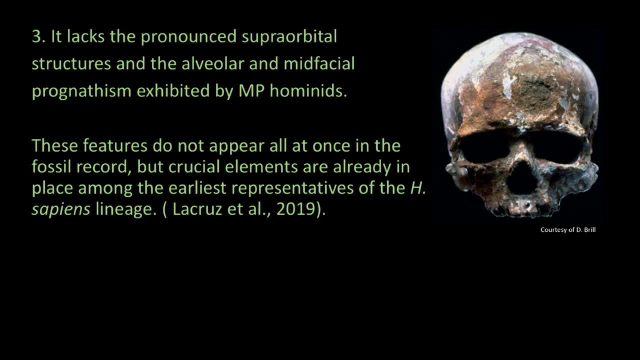 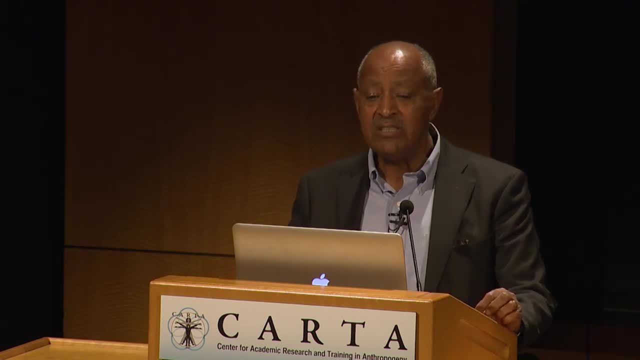 in place among the earliest representatives of homo sapien lineages. This presentation will focus on hominid fossils. I'm using hominids just only for those who are bipedal. My hominid definition does not include chimps and gorillas. 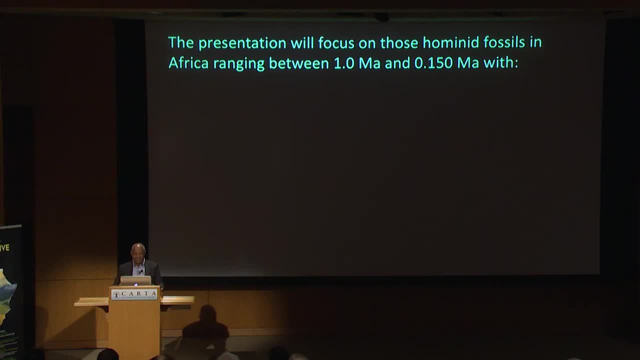 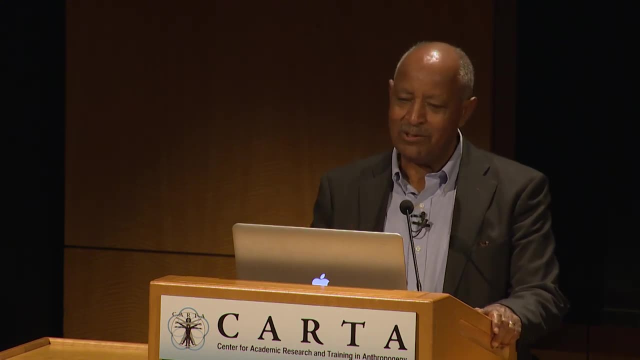 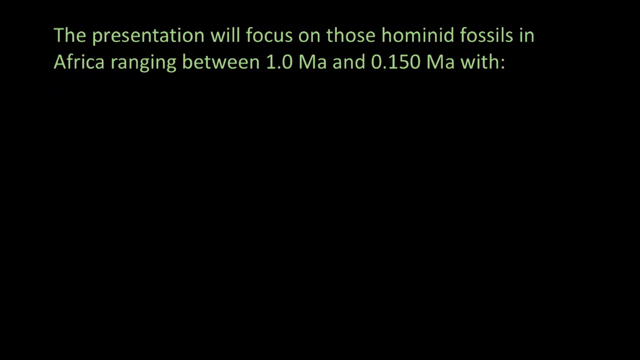 I'm talking only about the bipedal ones. okay, Because the recent classification used hominin. I'm not using hominin, I'm using hominid. Hominid is bipedal for me. okay, This presentation will focus on those hominid fossils. 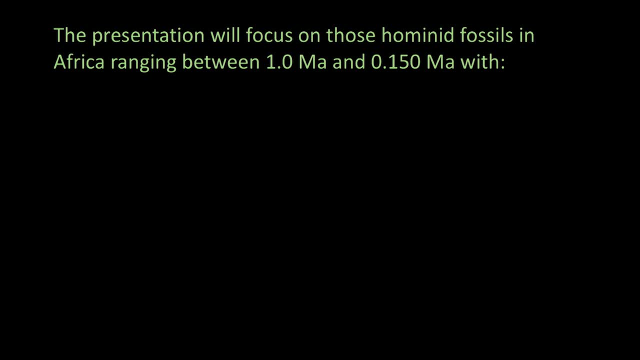 in Africa ranging between one million years and 150,000 million years. The reason why I do that is one they have to be. they have to have good stratigraphic hygiene. I use the word hygiene because usually it is. it's a mess. 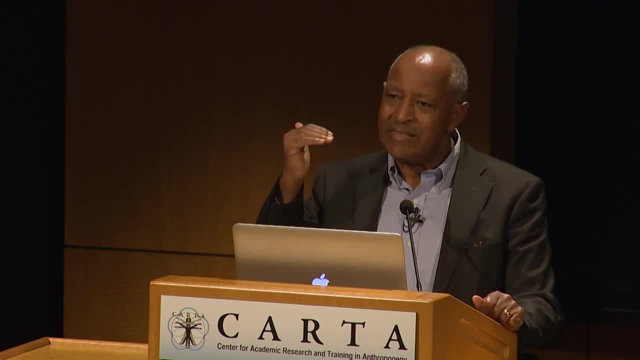 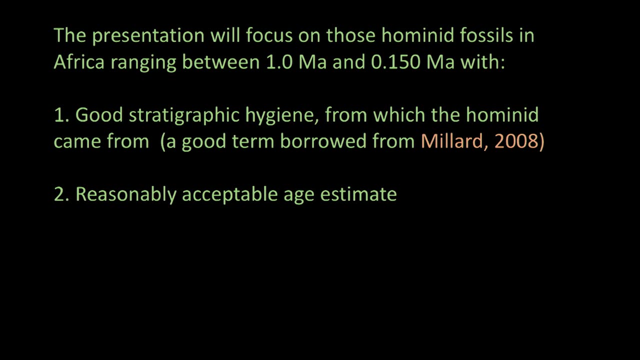 They have to be clean, they have to know exactly where they came from. This is a word I borrowed from Miller in 2008,, which is a very important word, and the other thing is the age range. The reason I'm using age is: 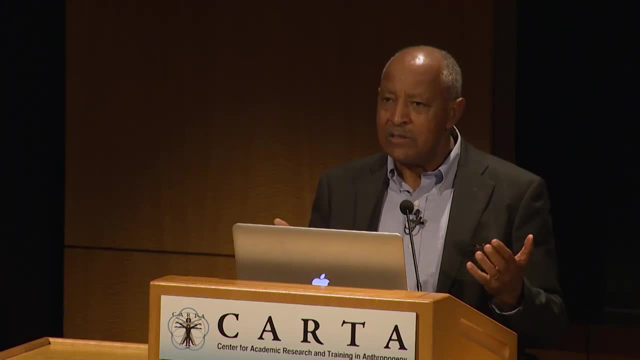 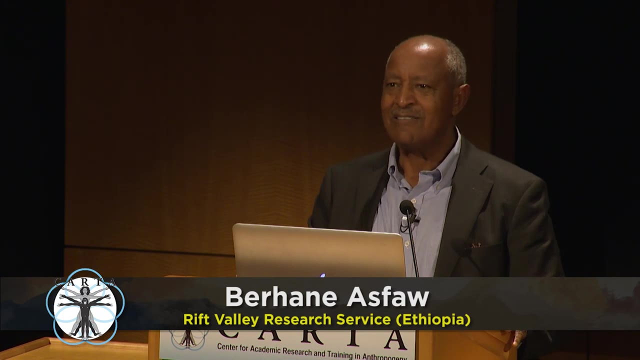 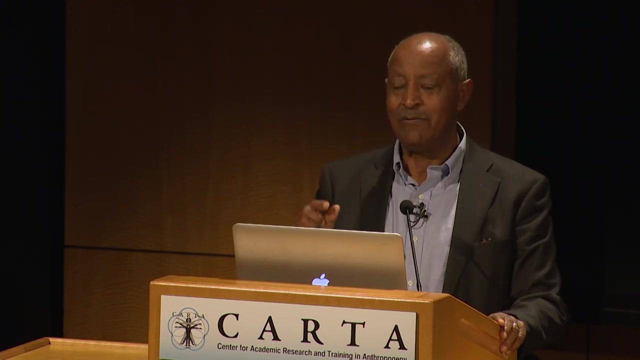 there is reasonable, acceptable age estimate, Because the age range of some of the fossils that we are dealing with these days are just enormous. But we prefer a certain age. Sometimes we prefer it's not because that's the age that is the preferred age. 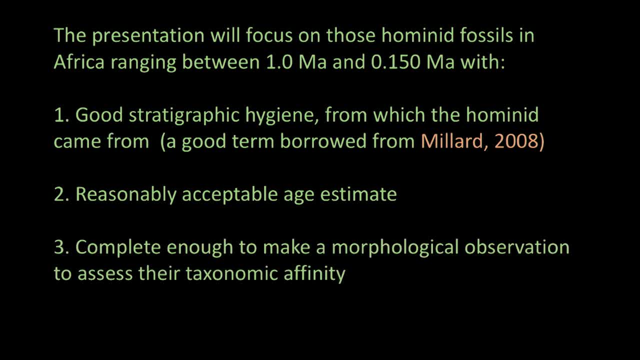 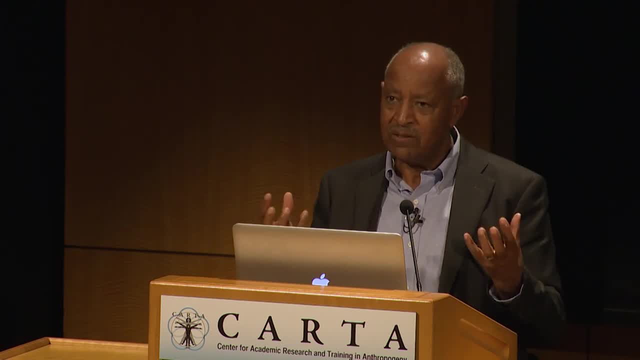 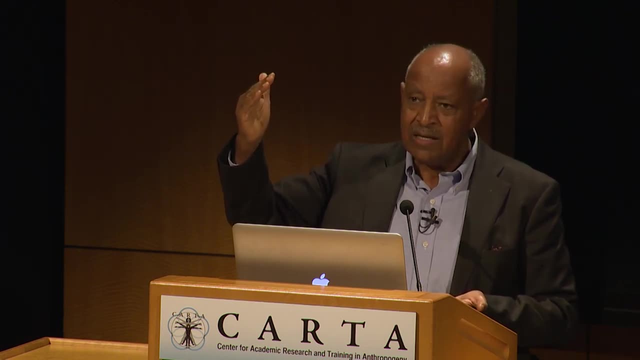 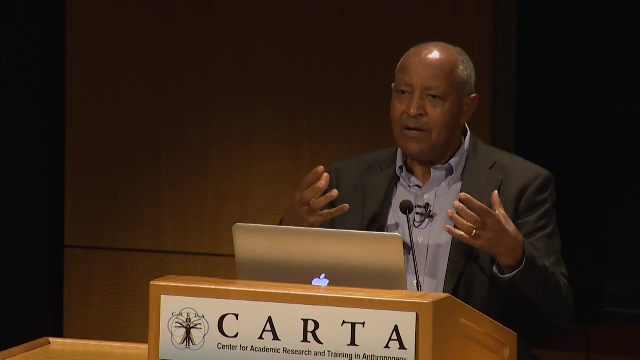 which is scientifically unacceptable to assess their taxonomic affinity. So there are so many fragments of bones, of hominid bones ranging between one million years and 150,000 years, but most of them are just bits and pieces. So to make this assessment, I really want to use 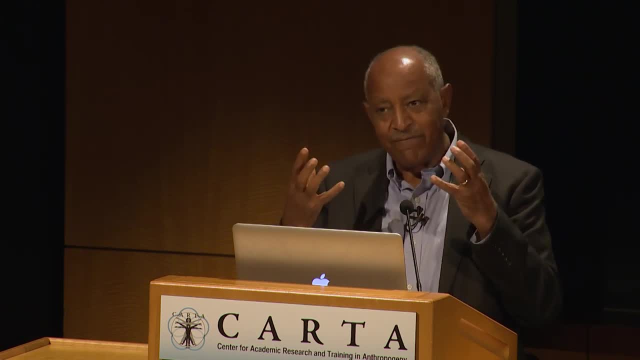 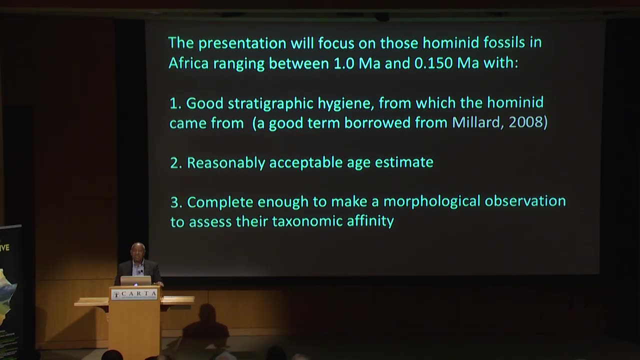 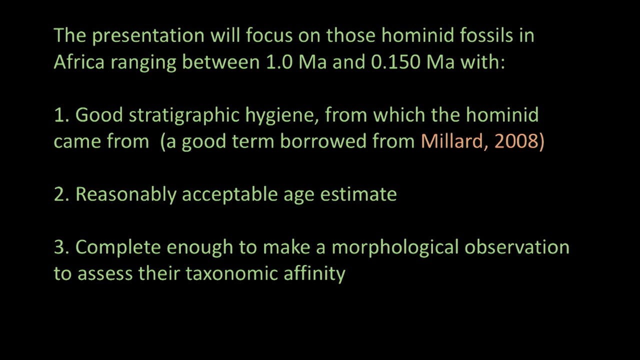 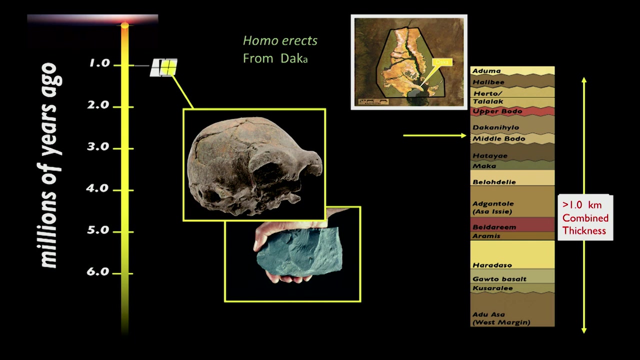 only those who do have mostly face face included and the other parts. So when I choose that there are so few in Africa, very few- I used as base, as a one million base level. I used the fossil that my colleagues and myself 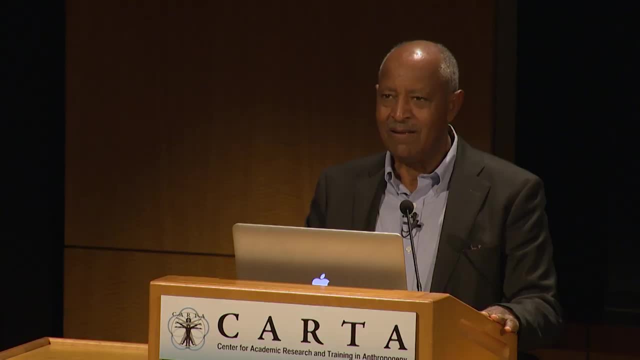 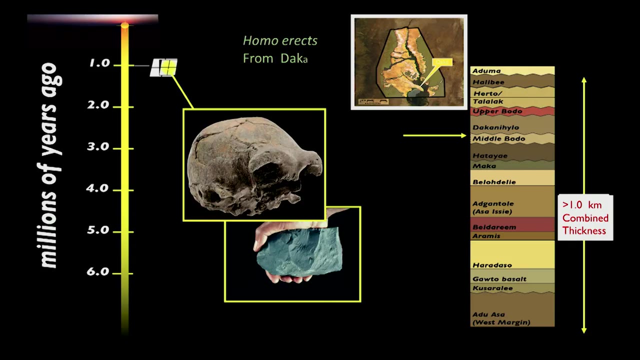 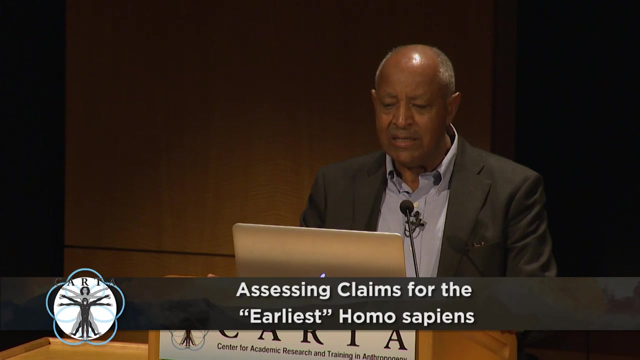 found from Mir Lawash, Dhaka, because I am 100% sure about its stratigraphic hygiene. It is clearly found from one million years ago, based on Argon-Argon dates and the stratigraphy is clearly labeled. So, with this understanding, between one million. 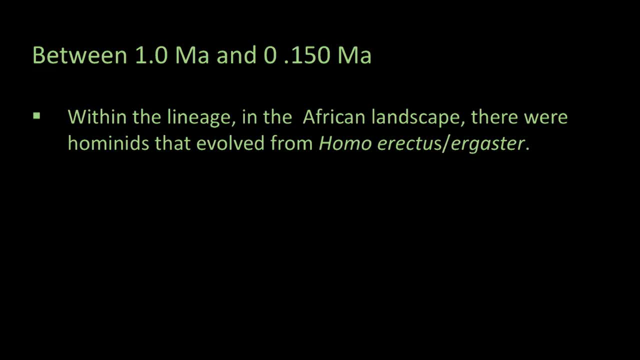 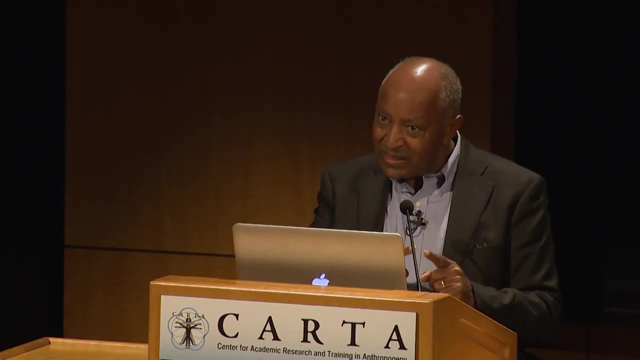 and 150,000 years ago, within the lineage in Africa, the African landscape, there were hominids that evolved from Homo erectus or whatever you call it, Homo regaster. Some people prefer that There are hominids of the lineage. 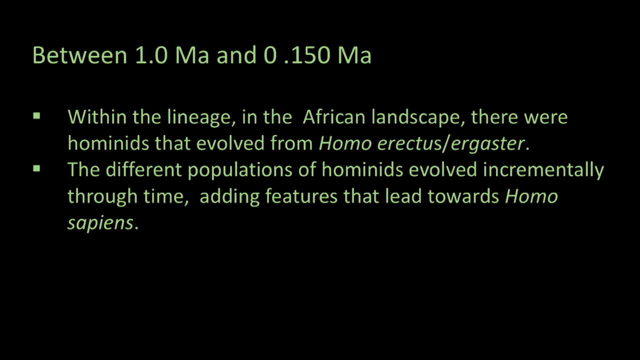 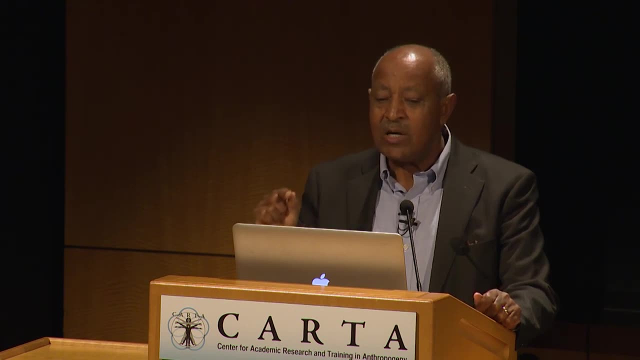 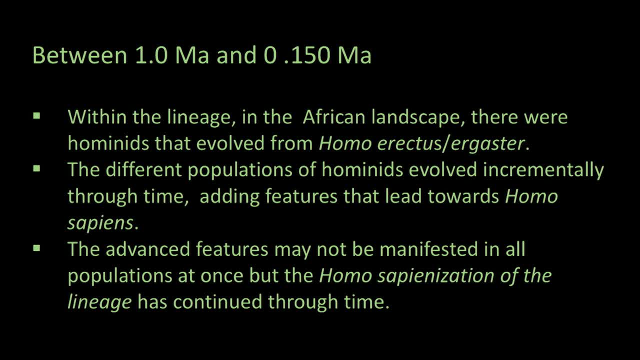 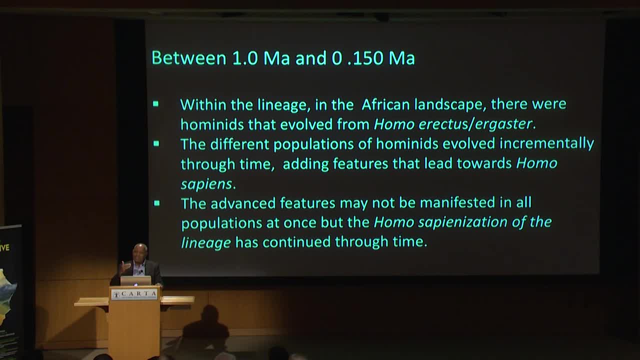 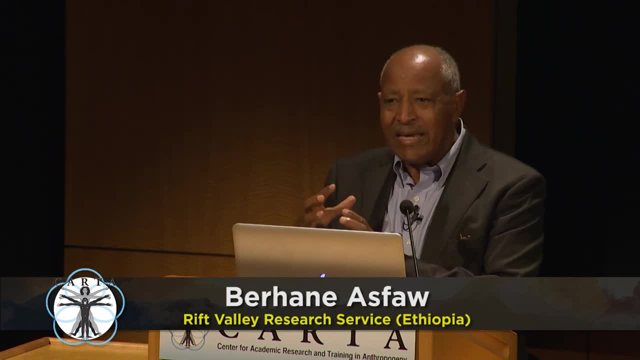 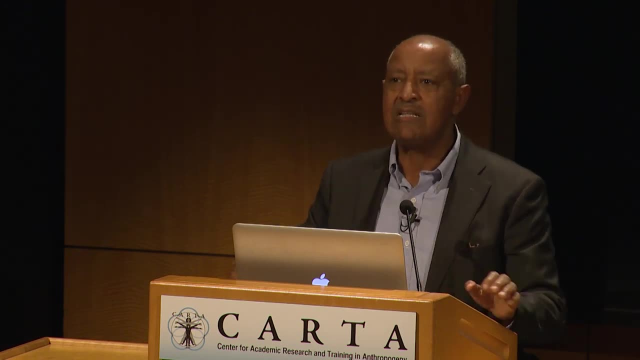 So I see the lineage. it's not didn't appear, meaning the Homo sapiens package did not appear at once. It is a process. It increases character through time. That's what I see in the fossil record. Then my base- the top is what I used- is Homo sapien adulto. 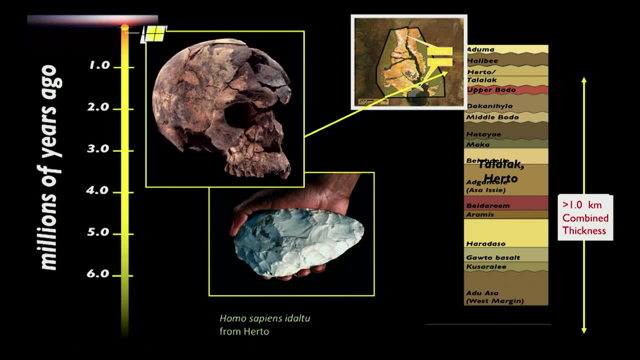 This is another one which I'm 100% sure about its stratigraphic hygiene, which is 150, between 150 and 160,000 years boundary, And the age is undisputable. So the morphology it has a clear Homo sapien morphology. 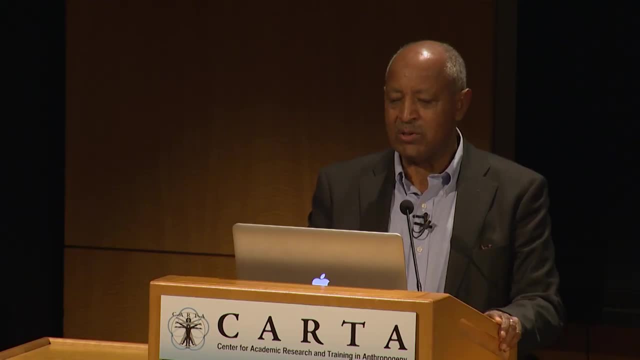 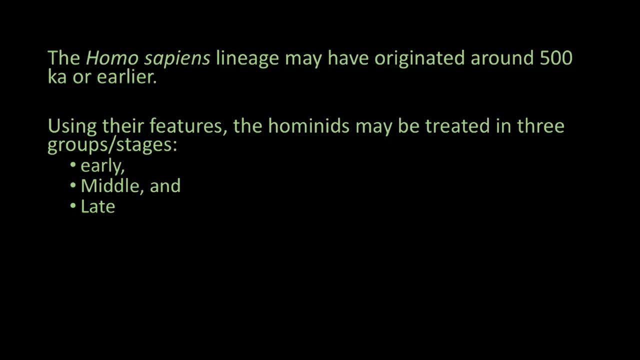 around 500,000 years ago or earlier. So, using this their features, the hominids may be treated in three groups or stages: Early, middle and late stage. This is an arbitrary boundary that I try to break. them The earliest. 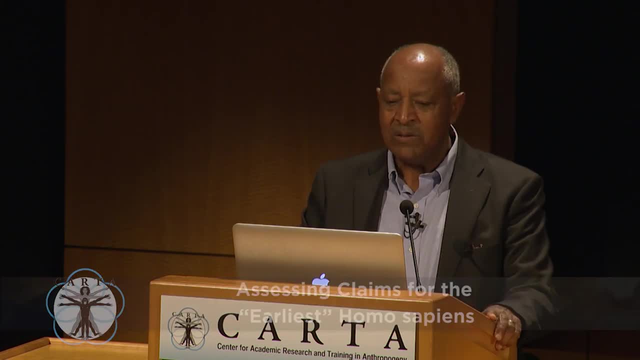 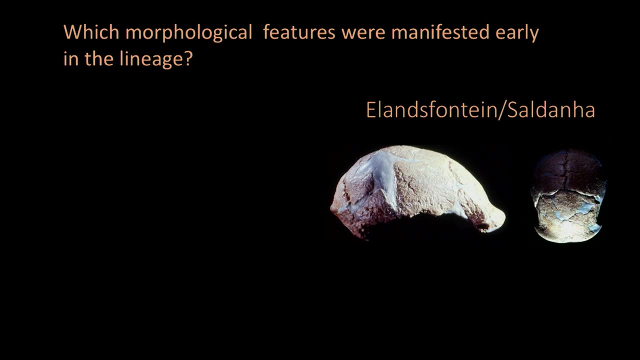 This is an arbitrary boundary that I try to break them From the complete ones, which is part of the face, Which is the morphological feature that we that were manifested early in the lineage is from Ellen's Fontaine Saldana. 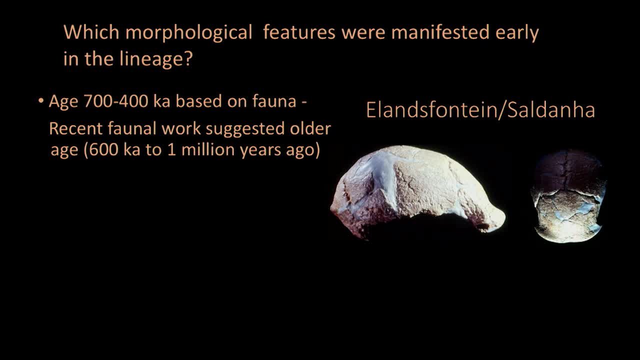 The age between 700 to 400,000 years ago, based on fauna. Recent fauna work suggested older than 600,000, maybe from 600 to 1 million. The brow ridge is. this is what we call the brow ridge. 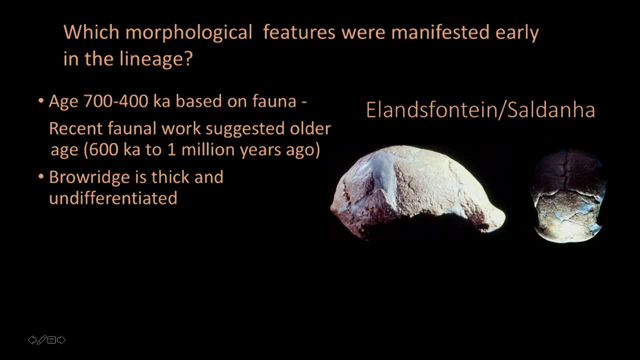 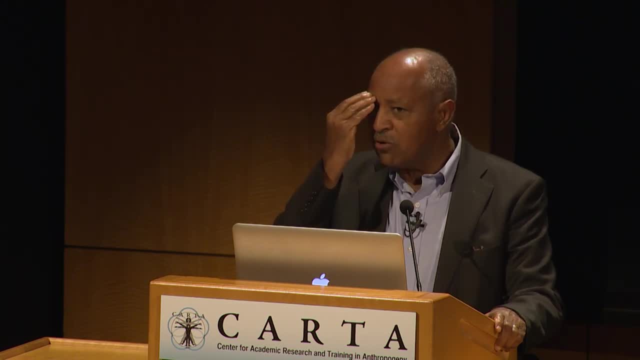 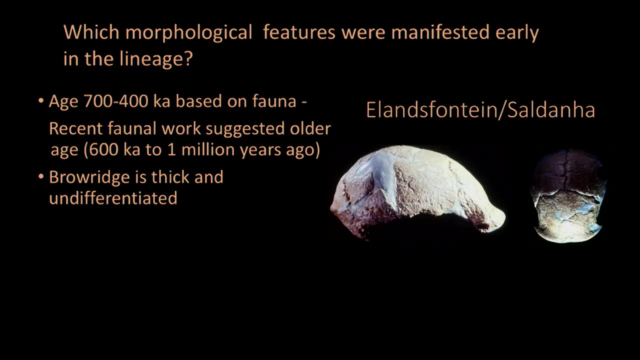 The brow ridge is very thick and undifferentiated- Undifferentiated means in Homo sapiens- the middle part, which we call the supercellular part, is a little bit thick and the lateral part is thin, But in Ellen's, Fontaine or Saldana. 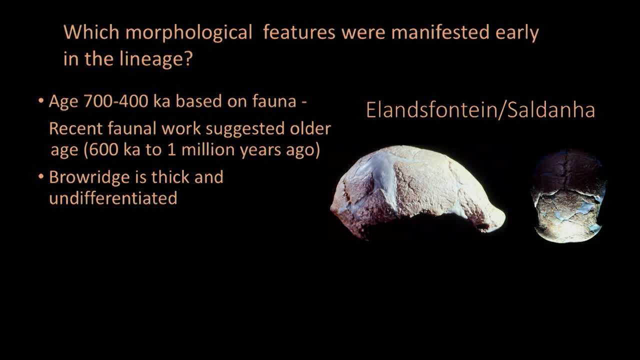 it's thick mediolaterally, which is a very primitive feature. The occipital torus is not strong and that is common to all Africans, African, even African Homo erectus. they all have similar kind of. we cannot use it. 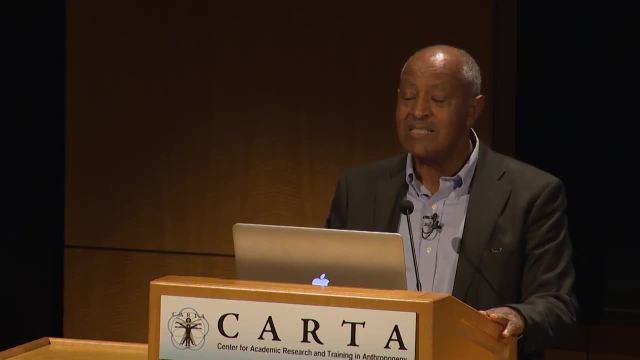 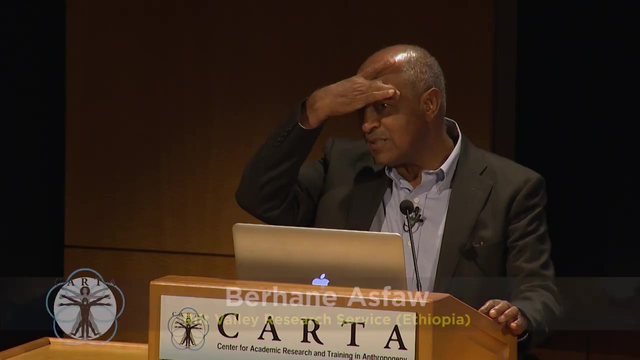 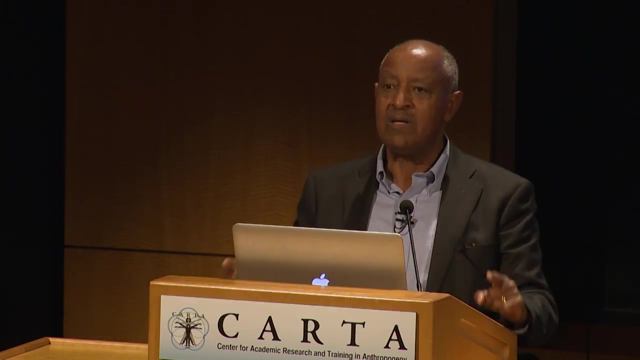 But what else do we use? The frontal is less constricted. This is the beginning of Homo sapienization. The frontal part. this part is not constricted In the earlier parts, in the earlier groups, in Homo erectus. this is the lateral part of the most 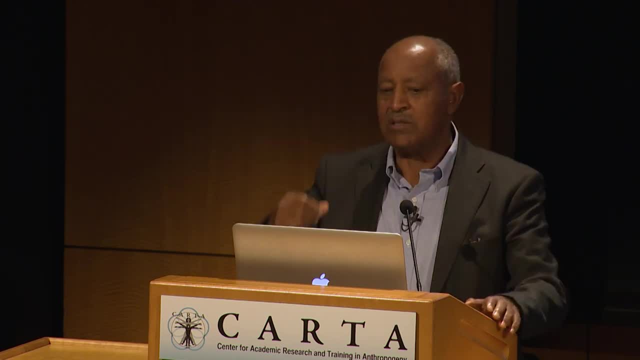 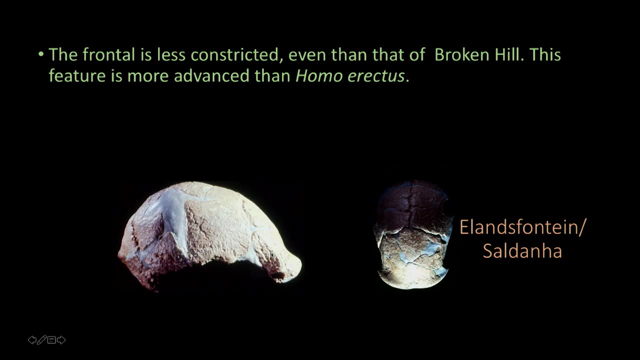 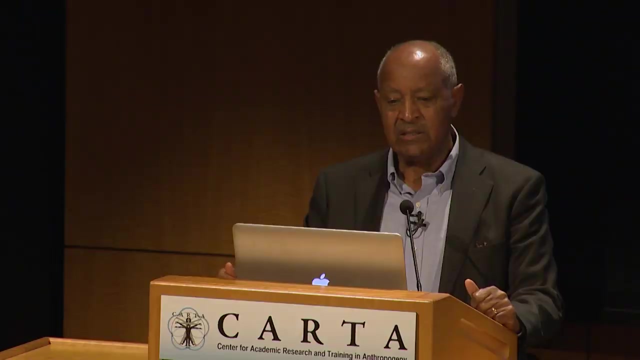 lateral edge of the brow ridge is very wide compared to the frontal, But in this, in Ellen's Fontaine, the frontal is not very constricted. It's even less constricted, even than that of Broken Hill. This feature is more advanced than that of Broken Hill. 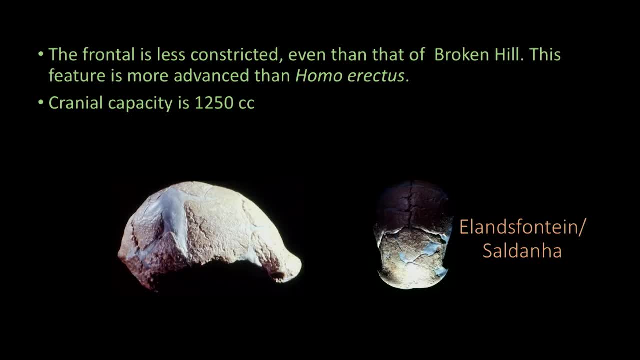 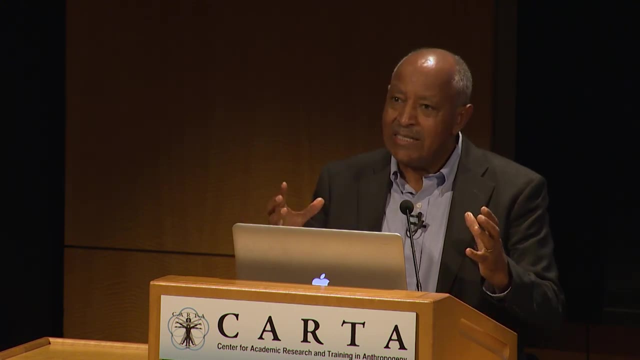 This is more advanced than Homo erectus. This is a beginning, And the cranial capacity is 1,250 cc. It's much bigger than Homo erectus. Much bigger than Homo erectus. That means brain expansion has started. This is a trend going towards Homo sapiens. 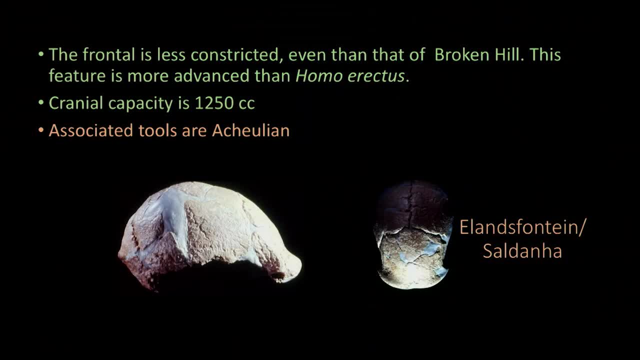 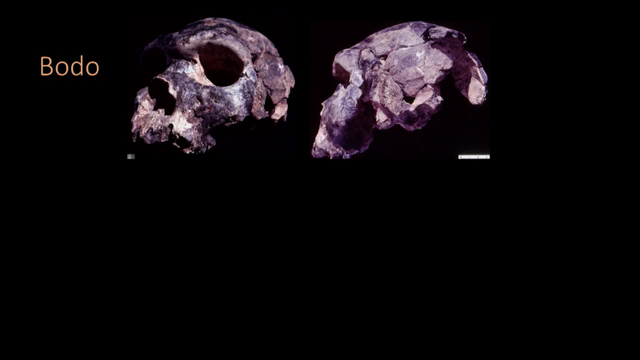 Okay, then the associated tools- still Lachullion. That is the kind of tools that we have been seeing with Homo erectus. Let's go to the next group. This is Bodo. Bodo is skull found in the middle awash. 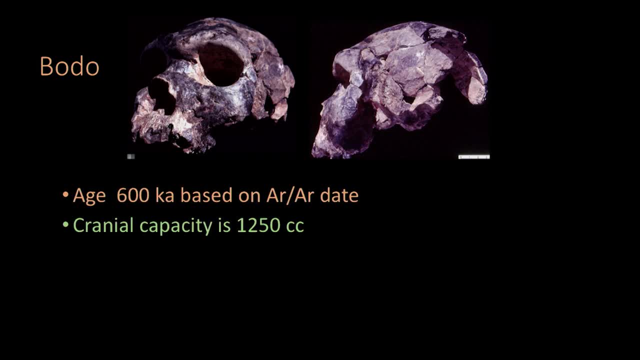 in the area that I have been working in the last 30 years. Age 600,000, based on Argonaut bond dating, Cranial capacity is exactly the same as Ellen's Fontaine or Saldana. 1,250 cc. 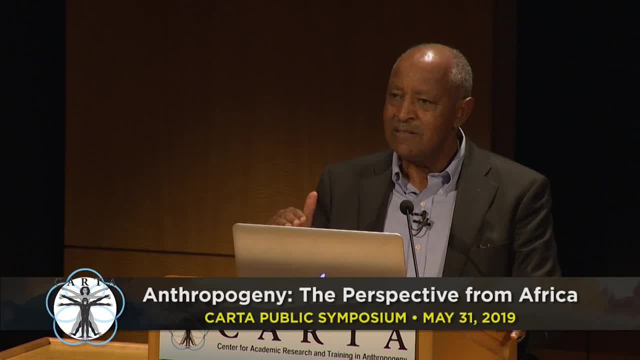 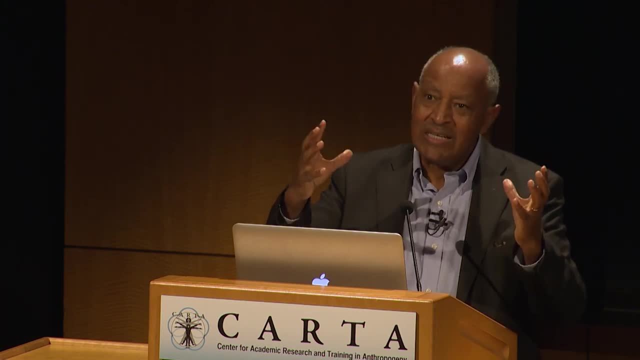 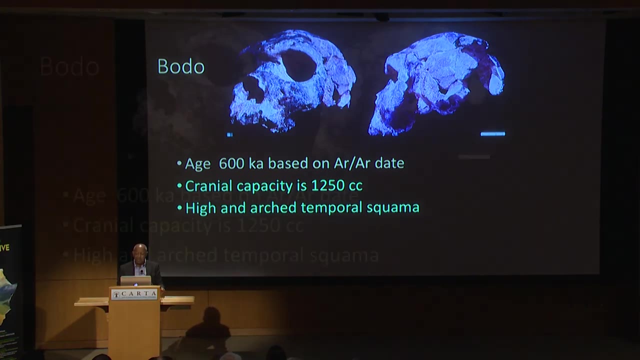 Much bigger than Homo erectus. The Homo erectus is under 1,000 cc. That means the brain has started expanding, Expanding, which is a direction that we see going towards Homo sapiens High and arched temporal scoma. 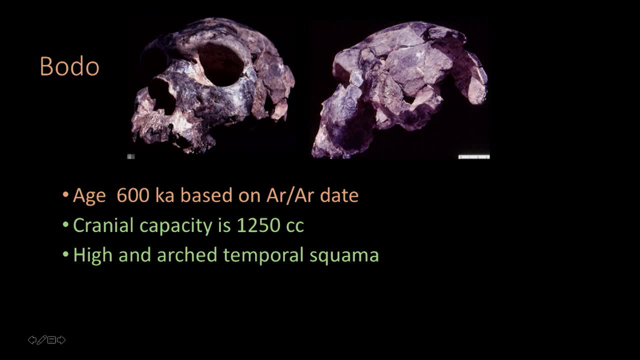 When you see this, this region, in Homo erectus it forms almost like a straight line, But in these guys it forms like an arch. It's an advanced morphology, Supraorbital torus, differentiated Meaning. the lateral part is thin. 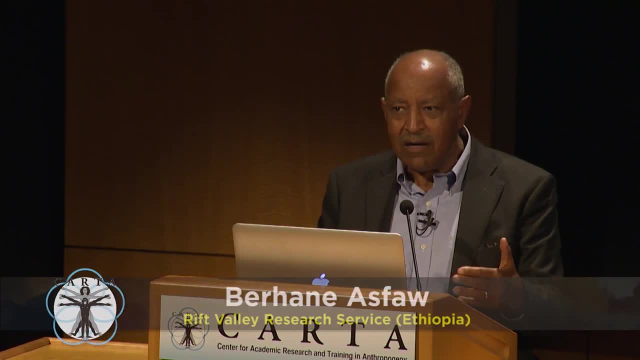 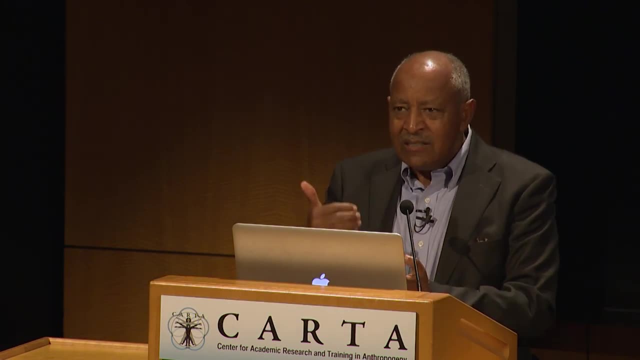 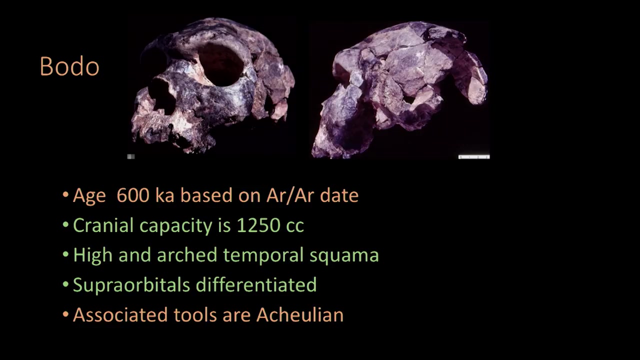 and the medial part is thick. This is a kind of morphology that we see in Homo sapiens. So that means they are adding morphology to you know, going towards Homo sapiens. The associated tools are Acheulean like Homo erectus. 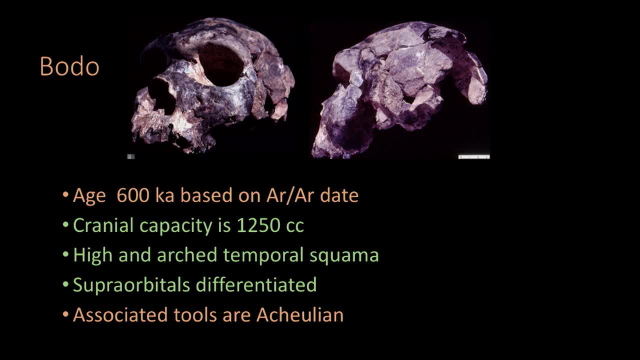 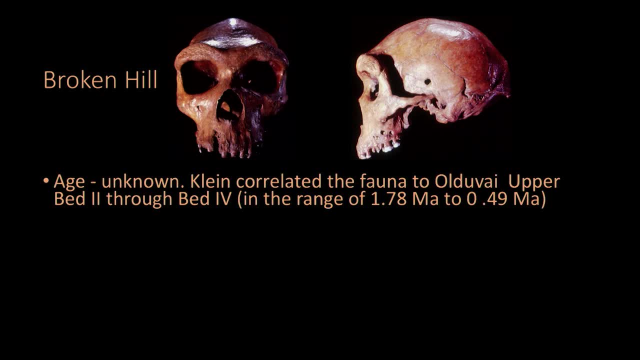 But the morphology is changing. Unfortunately, the occipital part is not preserved. Unfortunately, the occipital part is not preserved. Unfortunately, the occipital part is not preserved. What about broken hair? Age unknown, We don't know. 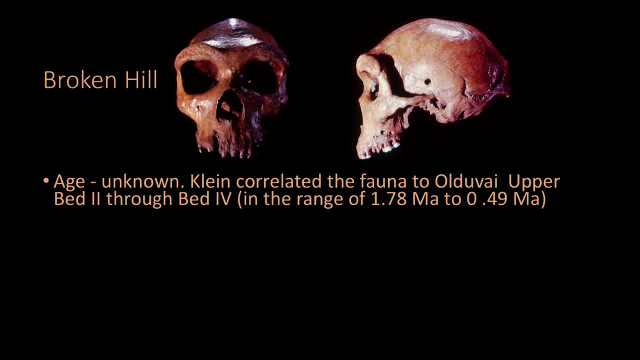 Klein correlated the fauna of Olduvai, upper bed two through bed four. That age range is between 1.78 to 490,000.. You can put it anywhere, But the temporal scoma is arched like Bodo. 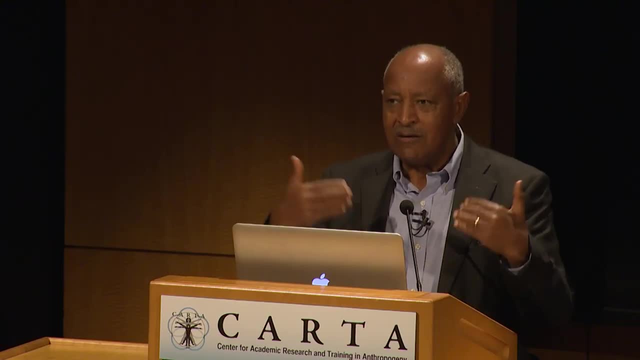 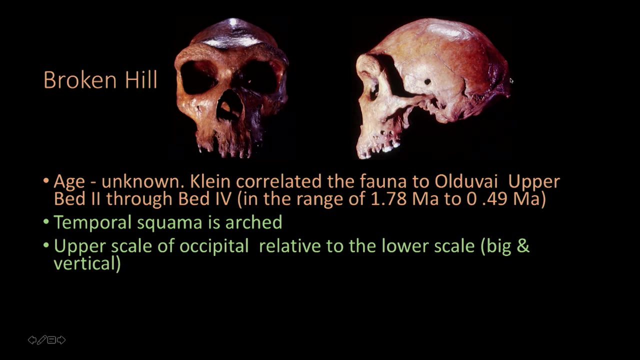 It's an advanced Homo sapien kind, Homo sapienization that we see. The upper scale of the occipital, which is this one, is relative to the lower scale, is big. That is also an advanced feature. Frontal is transversally expanded. 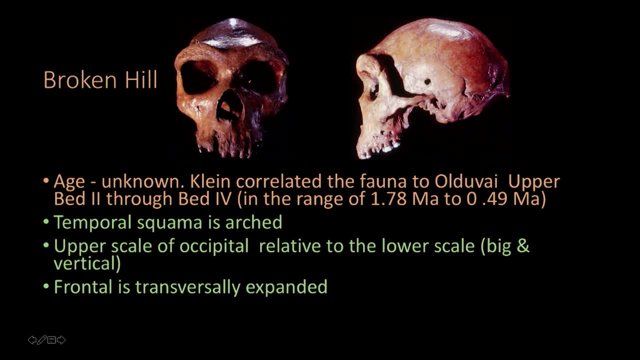 This is what we call the frontal. Unfortunately, it's still primitive because it doesn't have a forehead. We have a forehead which makes a difference from Homo erectus. We have a forehead which makes a difference from Homo erectus. We have a forehead which makes a difference from Homo erectus. 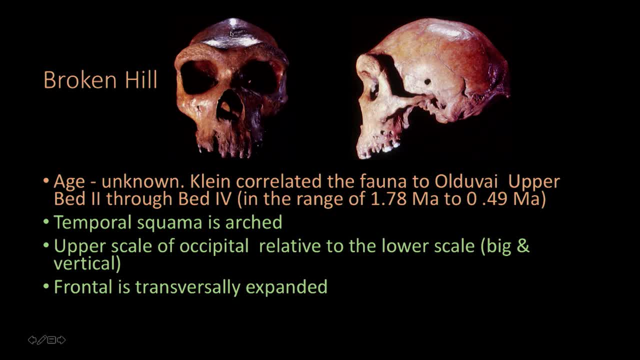 But this guy, even though he has big brain but no frontal yet, but still transversally expanded, It's big, It's a Homo sapienization that we call A cranial capacity, is a little bit bigger than Bodo and Saldana. 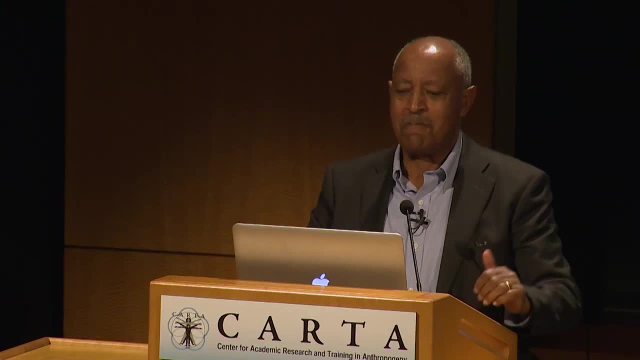 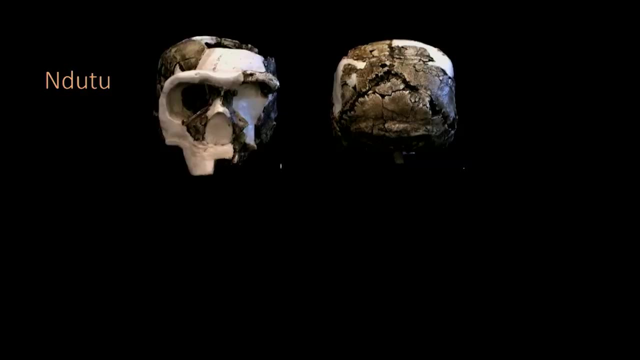 Now you can see the brain keeps expanding. The other features are not there. What about Ndutu from Tanzania? What about Ndutu from Tanzania? What about Ndutu from Tanzania? Age estimates: about 400,000 years old. 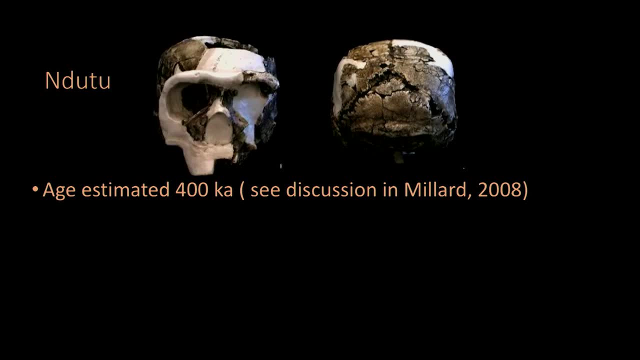 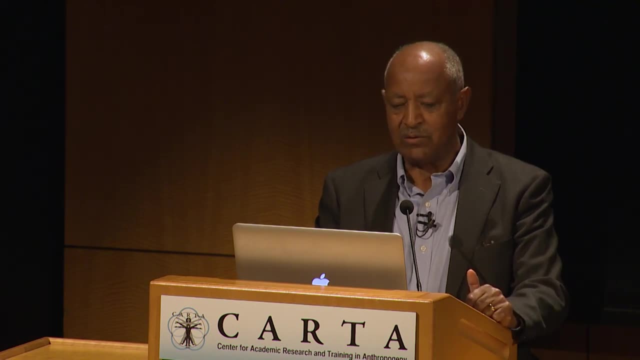 Age estimates about 400,000 years old: See discussion in Millard. There's so many discussions about the age, but about the age range is about 400,000.. What is important about this is cranial capacity, And so it is small. maybe a female. 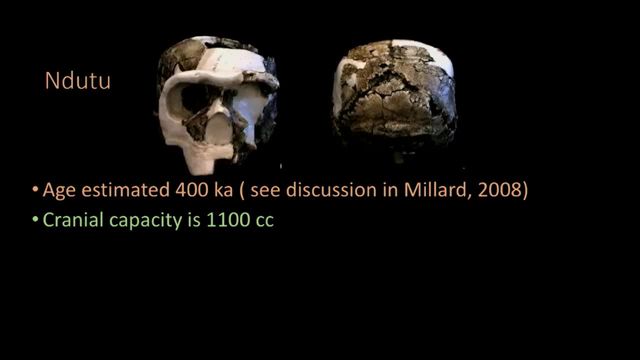 because there is a sexual dimorphism between males and females. One 1,100 cc looks smaller than Bodo Brockenhill and Saldana looks smaller than Bodo Brockenhill and Saldana. One 1,100 cc looks smaller than Bodo Brockenhill and Saldana. 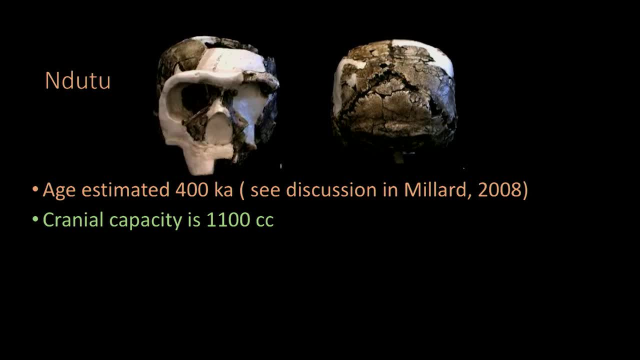 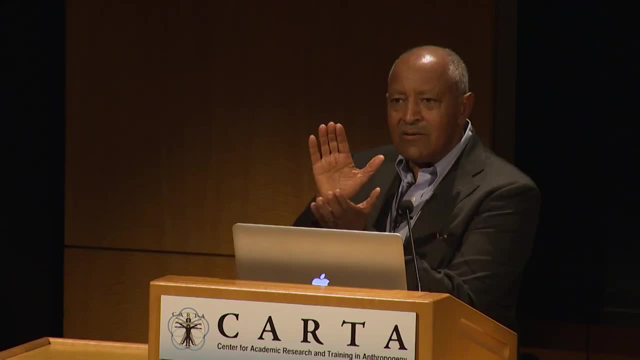 But it has more homo sapien features than them. But it has more homo sapien features than them. The occipital is not flexed. You can see it from here. It's an open occipital In Homo erectus it is flexed. 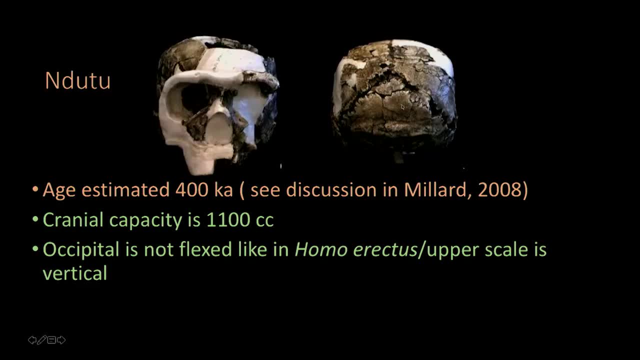 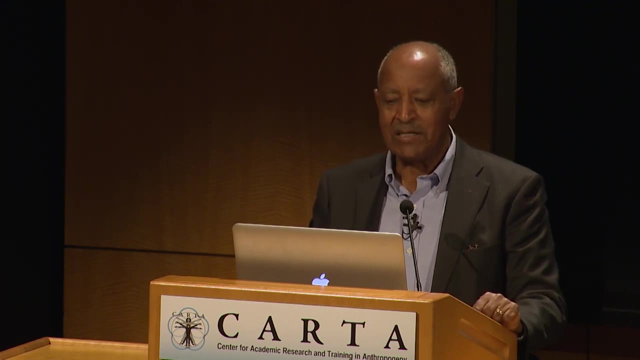 But this one is really open. Especially the backside is almost vertical, Has a post-canine fossa, something that we have never seen before, Either in Bodo, Saldana or Brockenhill. It is this part. We homo sapiens have a depression, right here. 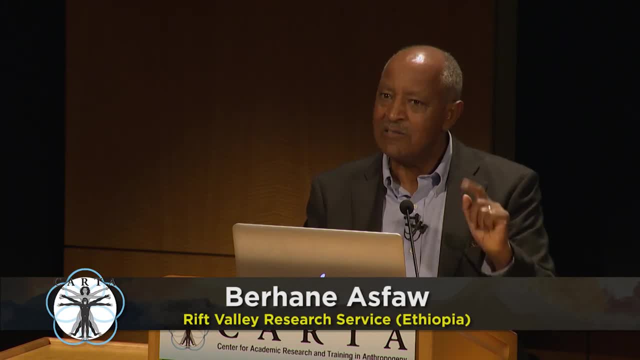 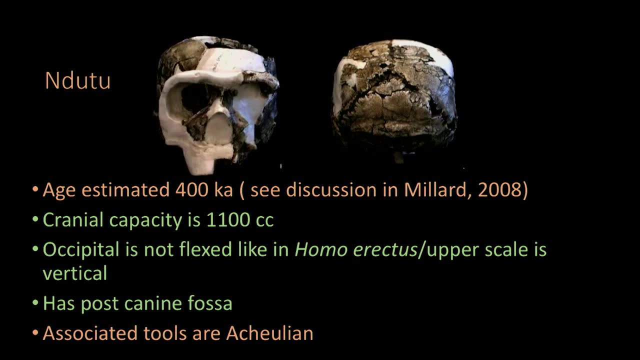 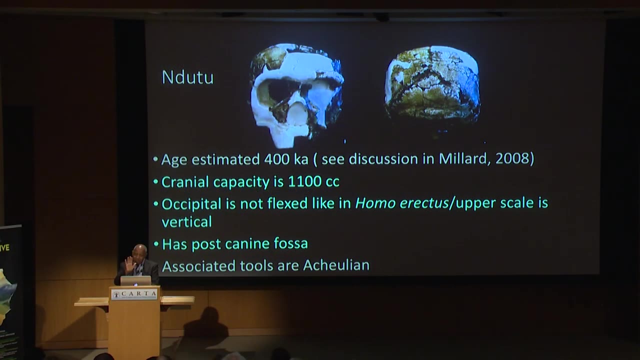 which we called the post-canine fossa, That is, homo sapien character. at that stage The associated tools still are Shulian, So the brain size is much more than Homo erectus. The occipital has changed towards homo sapiens. 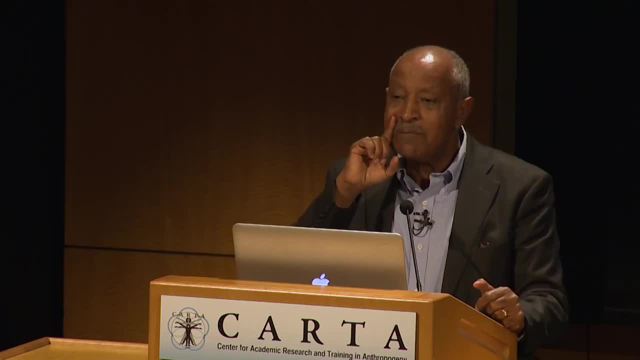 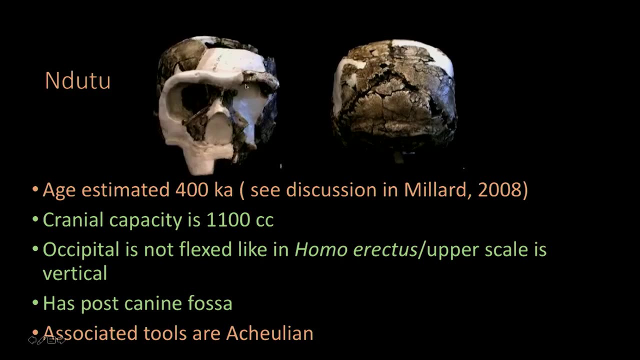 Vertical occipital, the upper scale, Canine fossa, the most important. the lateral part is developed And the torus is still thick. It shows a little bit of differentiation, but still the lateral part is very thick. It's a mosaic evolution that we see in these groups. 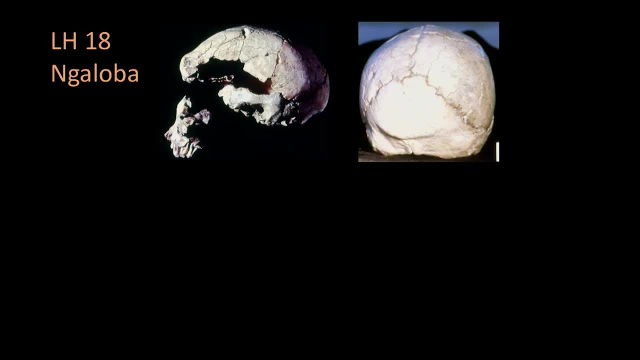 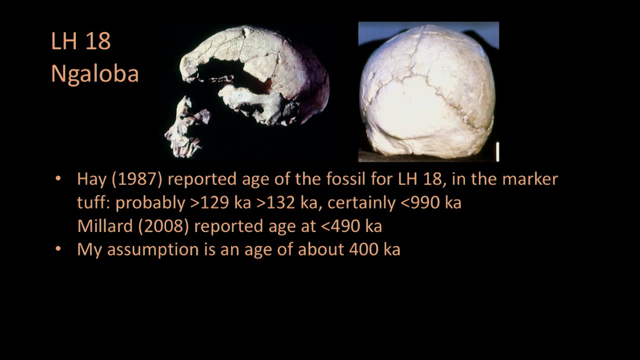 What about LH18?? Ngaloba again from Tanzania, from the Ngaloba beds. The age Hay in 1987 reported age of the fosso for LH18 in the markers. This is very tough, Probably greater than 128,, 29,000 to greater 132,000. 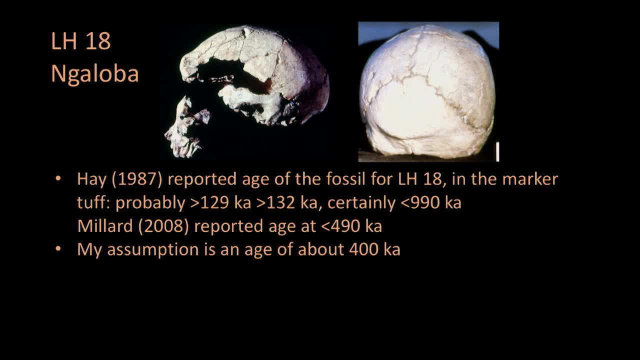 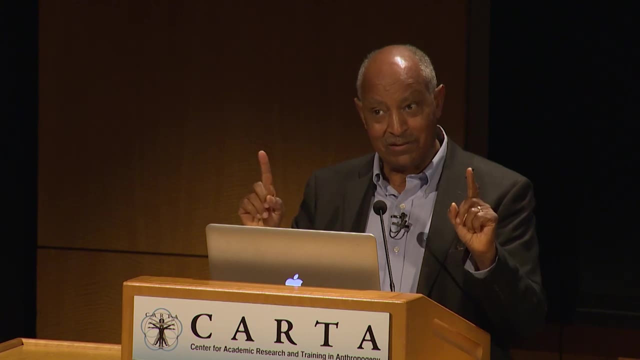 Certainly less than 990,000.. Millard 2008 reported an age less than 490,000.. Now you can see how messy the dating is. My assumption is an age of 400,000,. this is just an assumption. 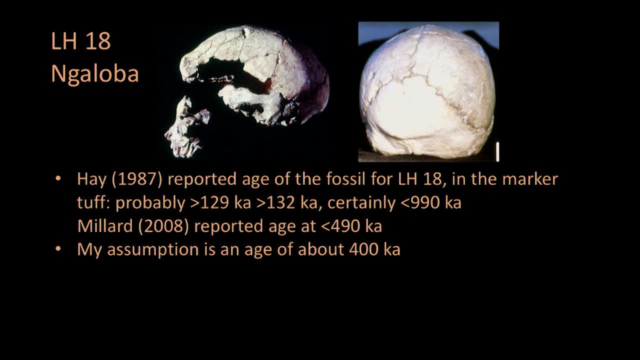 Maybe an age of 400,000 may be acceptable. Cranial capacity: 1,367.. It's big cranial capacity. Occipital: you can see the back of the skull open with no torus. That is also an advanced feature. 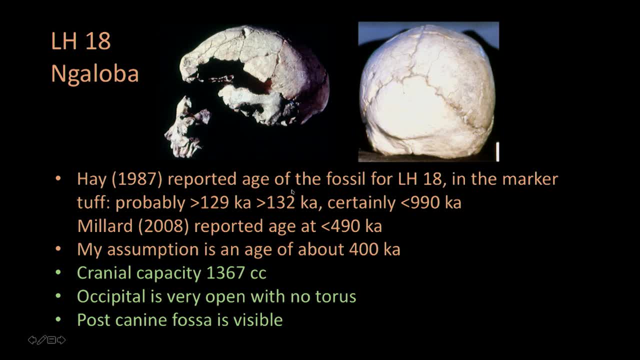 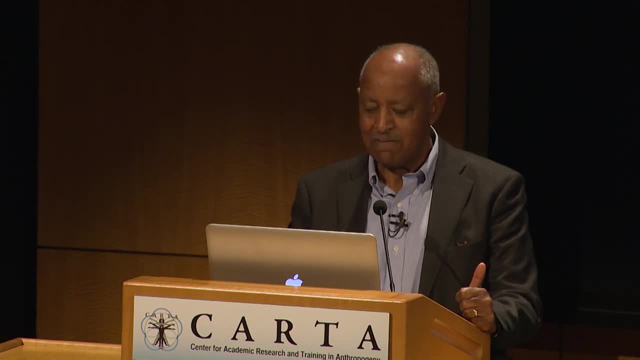 Post-canine fossa is visible, Like the one I showed you in the DUTU. it has a post-canine fossa which is also present in modern Homo sapiens like us. Okay, what about floor spat from South Africa? 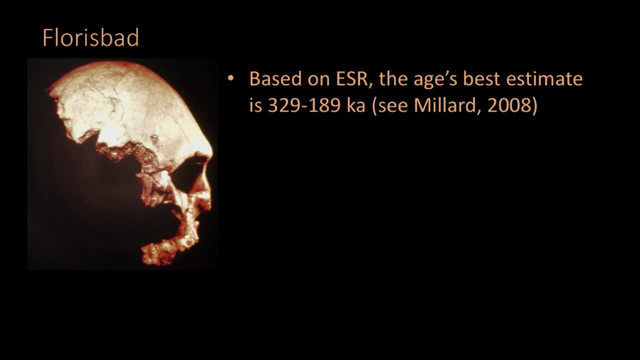 Based on ESR dates, the age's best estimate is 329 to about 189,000 years. similar in 2008.. Has a canine fossa. look at this. This depression is called the canine fossa- Short face typical for Homo sapiens, but the earlier form. 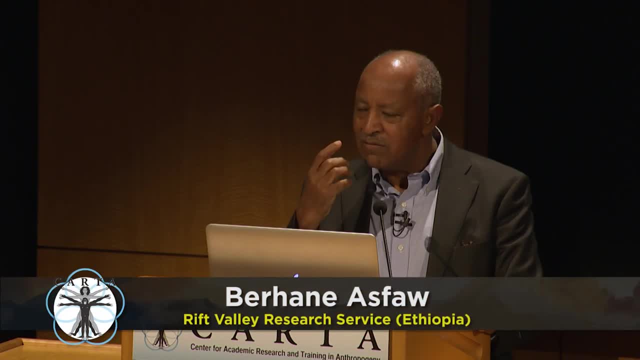 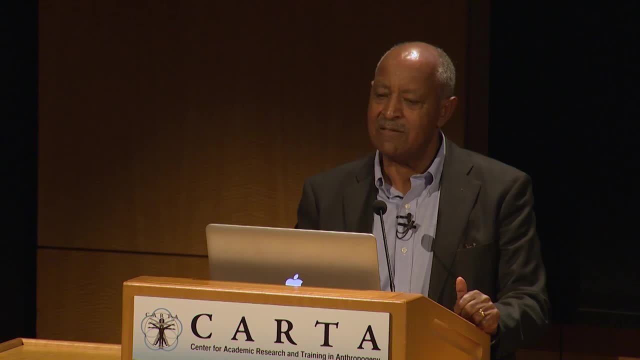 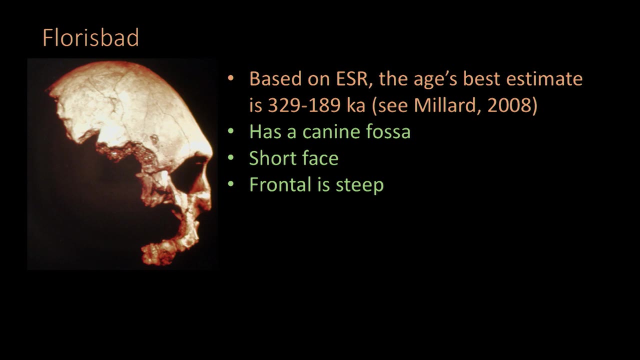 especially like Nogalova, the face is still big, even though it has canine fossa. That means everything did not come together. everything did not come together. Okay, the frontal is very steep. has developed a frontal steep frontal, a forehead. 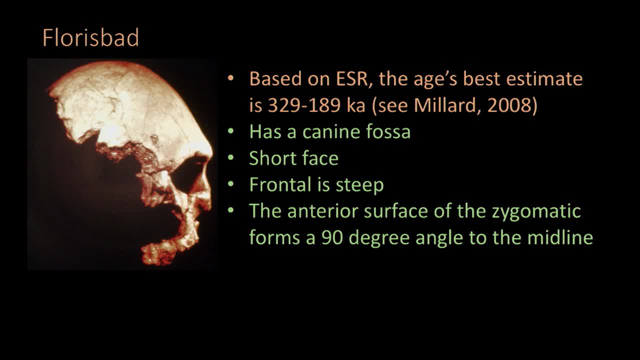 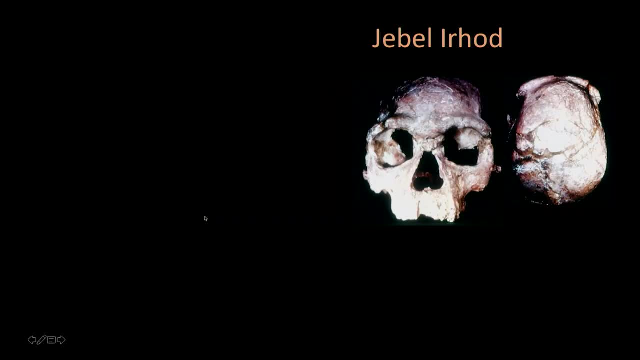 The anterior surface of the zygomatic forms 90 degrees. This one is 90 degrees. that is typical Homo sapien. What about Jebel Irhad? Long and low cranium, continuously thick brow ridge- These are primitive morphologies. 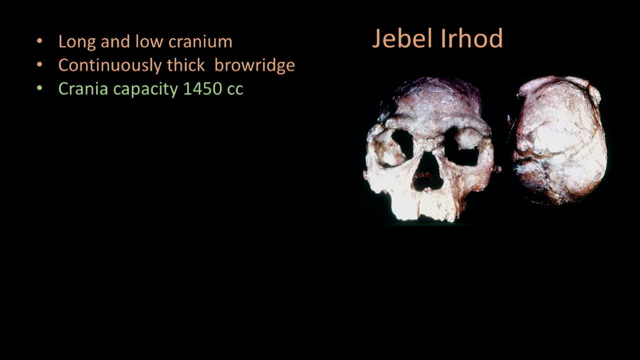 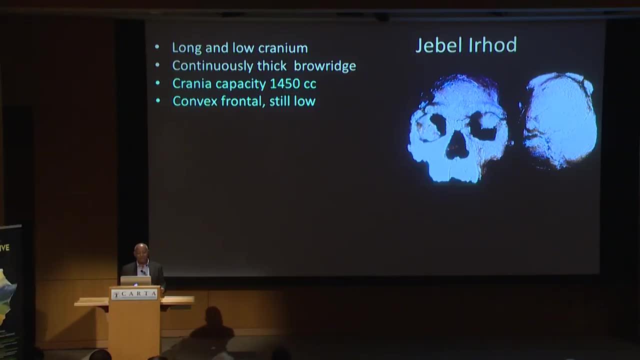 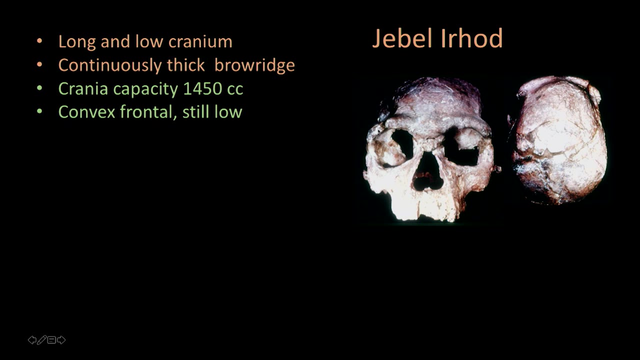 Cranial capacity is 1,450 cc. It's more than average even for modern humans. you know, Okay, convex frontal, but still low. Convex frontal, still low. Brow ridge is thick. medial lateral, which is very primitive. 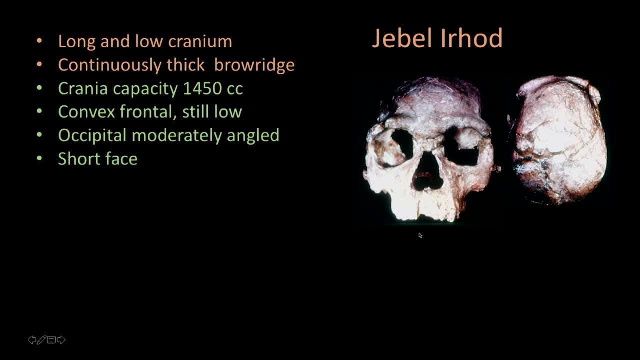 Occipital, moderately angled- Okay, Short face. The anterior surface of the zygomatic forms 90 degrees, which is typical Homo sapien. The dates of Jebel Irhad evolved from. it's an evolution of dates. now you can see. 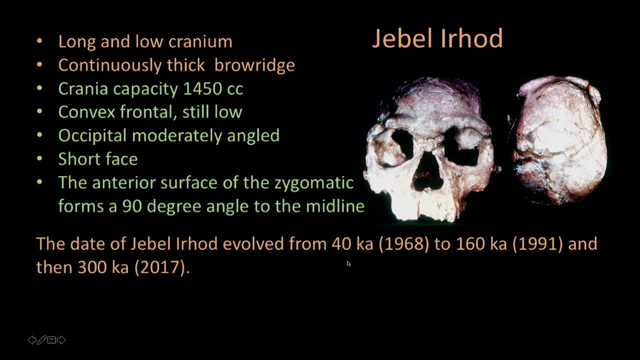 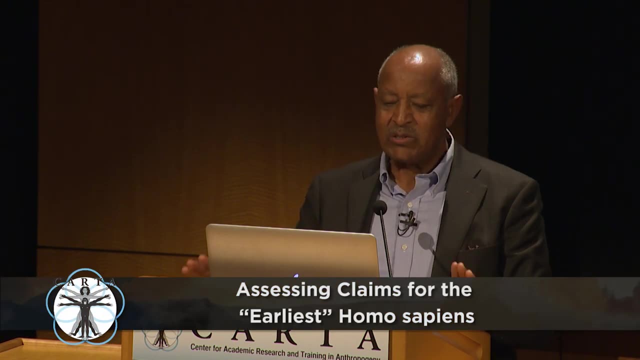 When it was first published, it was 40,000 years old in 1968, then 160,000 in 1991, and 300,000, 2017.. This is an evolution of dates. I suggest to re-date other sites like Floresbud and others. 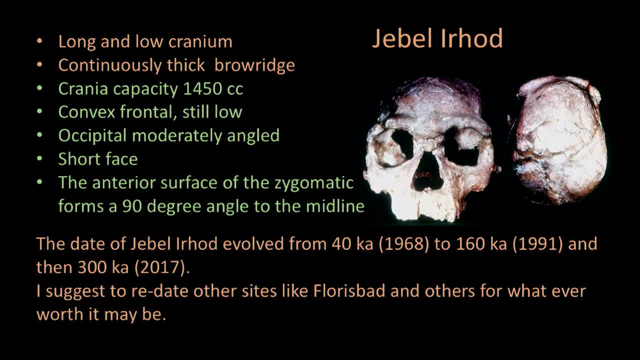 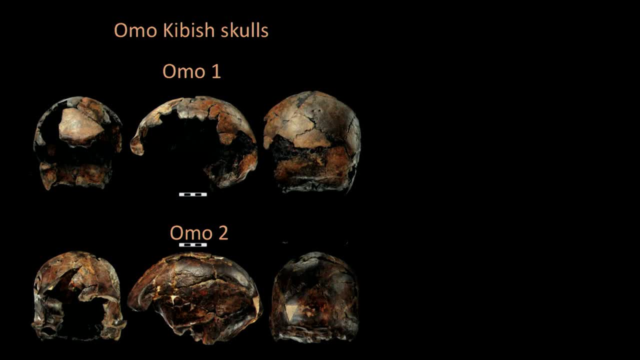 for whatever words it may be. If we re-date, they may also evolve in that direction. What about Omo, The Omo kibish skulls? there are two different kinds of skull. This is Omo I and this one is Omo II. 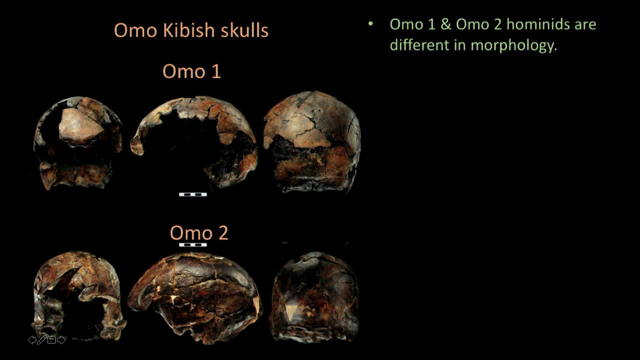 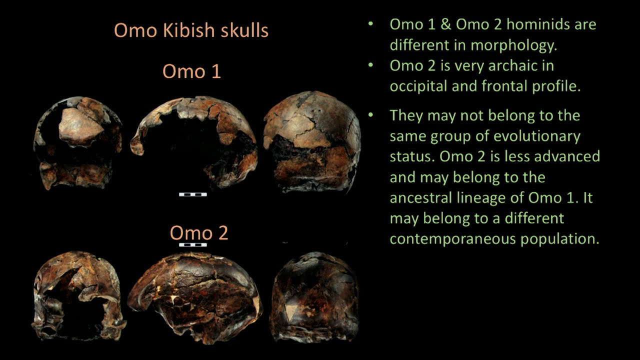 Omo I is very advanced, typical Homo sapien, Steep frontal occipital morphology, very Homo sapien-like. Omo II is very archaic in occipital and frontal profile. They may not belong to the same group of evolutionary status. 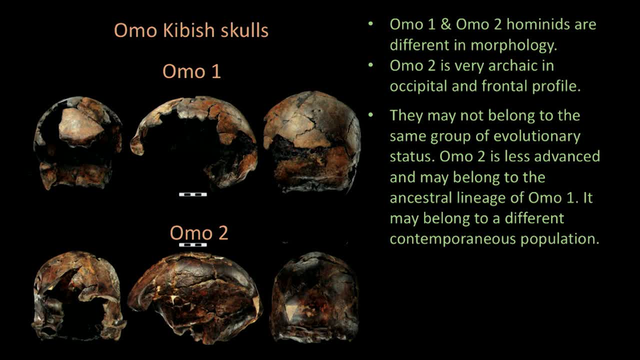 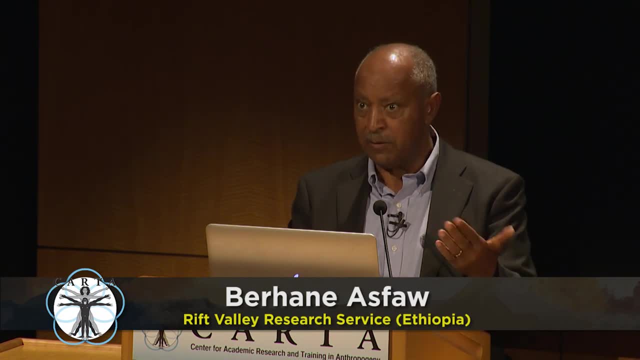 Omo II is less advanced and may belong to ancestral lineage of Omo I. It may belong to a different contemporary populations. It may If they, if they are from the same home. It may belong to a different contemporary populations. It may if they are from the same home. 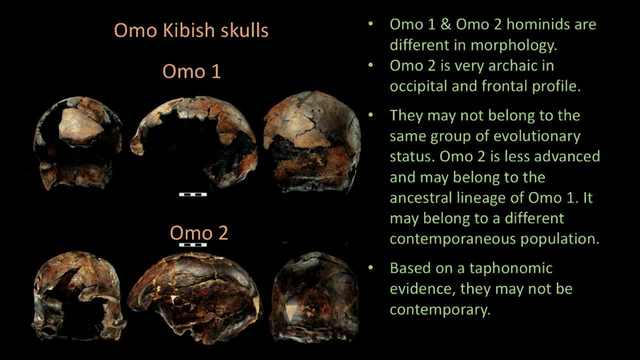 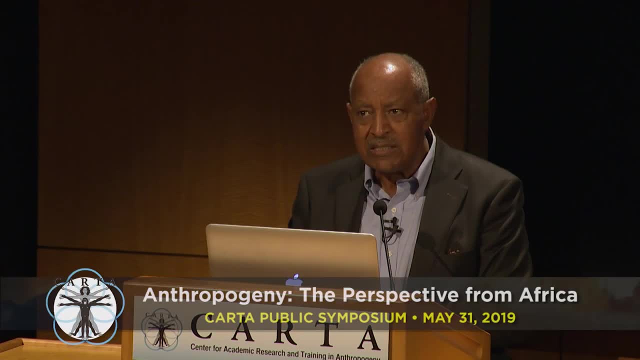 It may if they are from the same horizon. Based on taphonomic evidence, they may not be contemporaneous, Even though they are published as to be as contemporaneous for interpretation, it's misleading If we can confirm it. yeah, it's an evidence by itself. 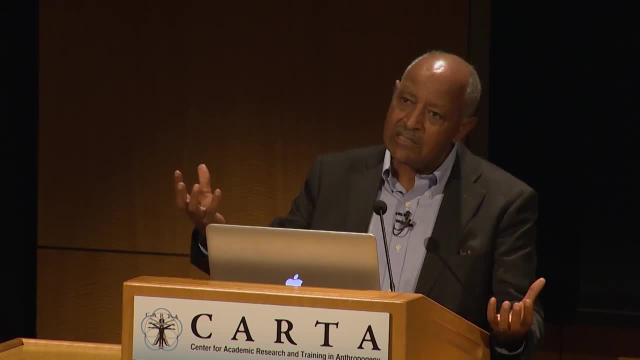 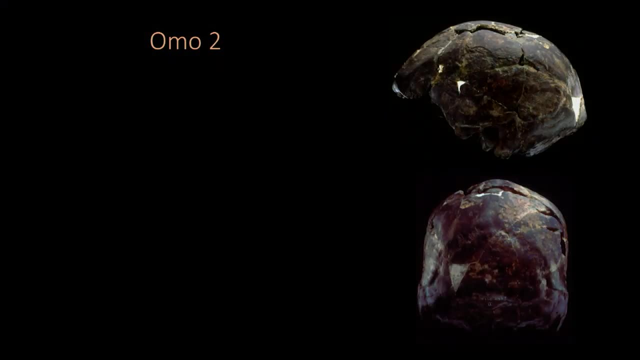 for two different populations, one advanced population, the other primitive population, to live side by side. But based on our observation, Omo II is very, very primitive. But based on our observation, Omo II is very, very primitive. You can see, it's an isolated surface. find: 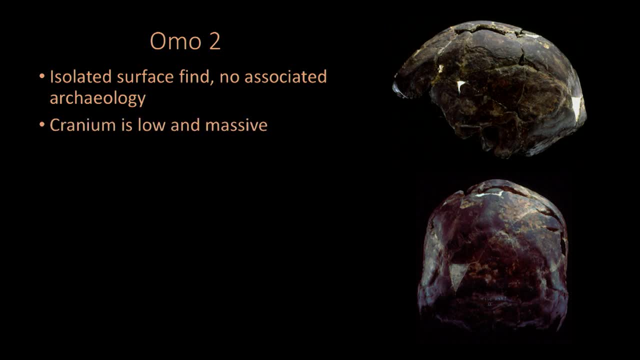 no associated archeology. like Omo I, Cranium is low and massive, very low, You can see. the frontal is very flat and the occipital is very flexed. unlike Omo I, Frontal is low, weakly keeled, strongly angled occipital. 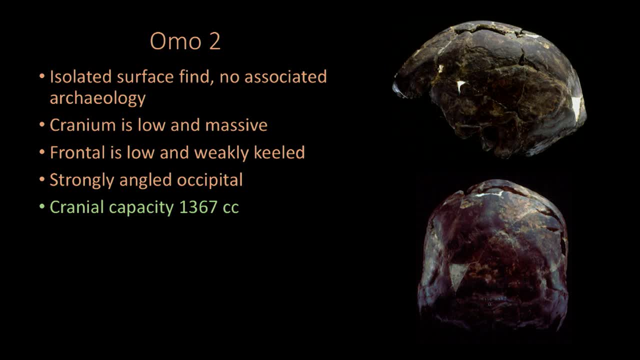 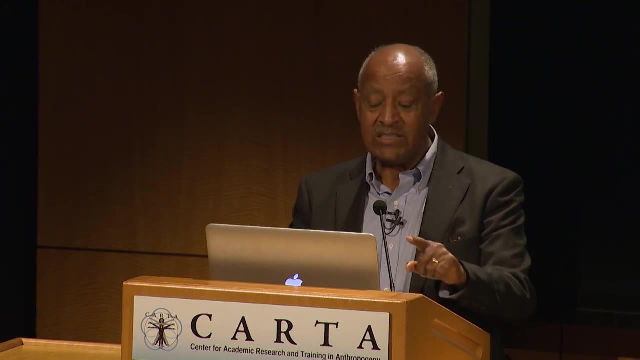 Cranial capacity is very big, typical Homo sapient type Broad and constricted frontal Broad and constricted frontal Parietal is bulged and expanded And it was a surface find, not associated stone tools. So we think based on this evidence that we observed, 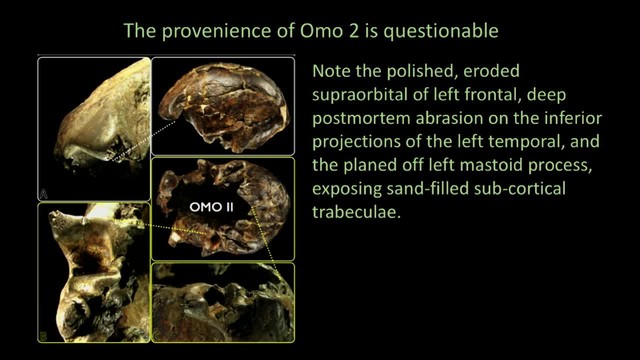 on the fossil, not the polished- eroded supraorbital. They are polished and eroded And the polish is also on the temporal surface. They are highly polished. So these features may suggest hydraulic transportation of the skull by Paleo-Omo river or its tributaries. 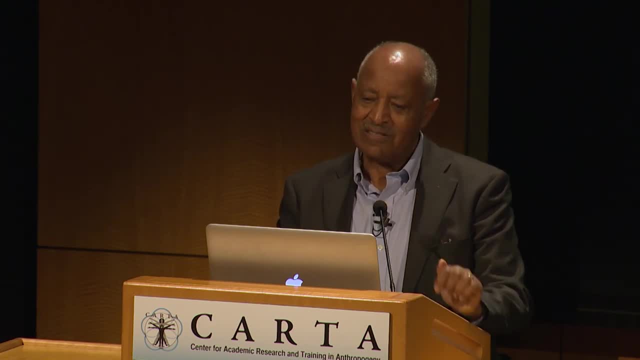 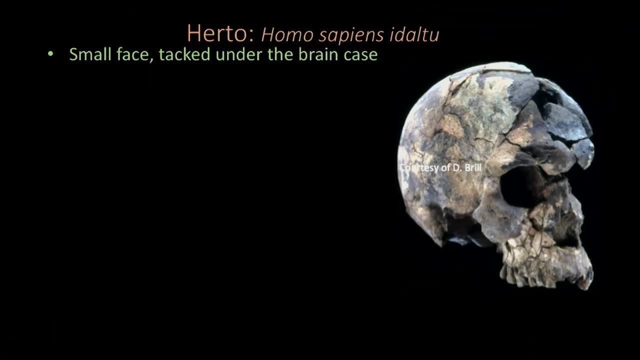 So I think they are not contemporaneous and this is a very good information to take into consideration. Hair toe. let's see: Small face tucked under the brain case. Small face tucked under the brain case. No projecting mid face. 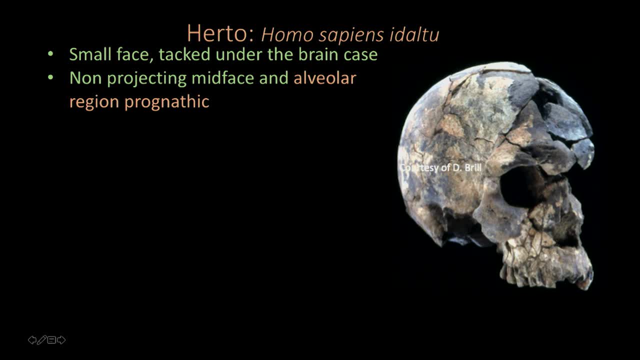 The mid face, not projecting, It's only there. The lower part of the face looks a little bit projection. It's a very, you know, kind of primitive character. Anterior surface of the zygomatic: this area forms a vertical orientation. 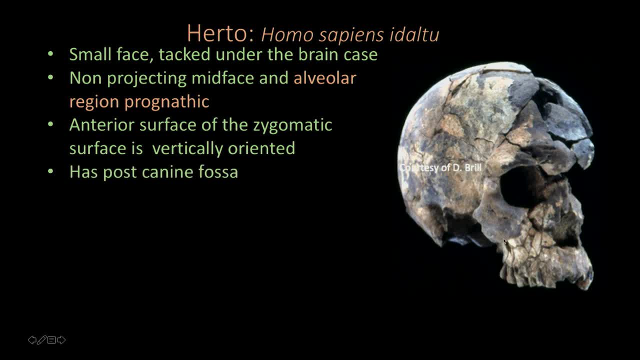 This vertical orientation, typical Homo sapient, has a postcanine fossa. that is something you have seen in nudutu and floresbud and jebel your heart, okay. Inferior border of the zygomatic joins 90 degrees. 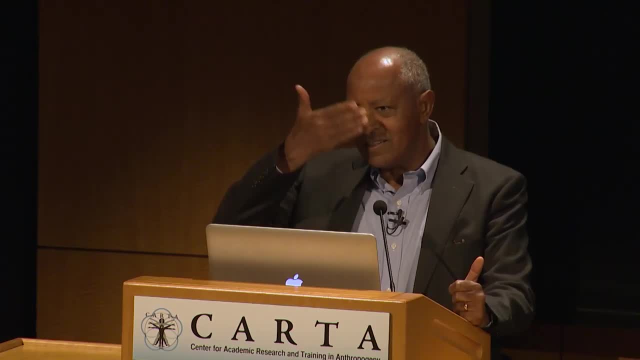 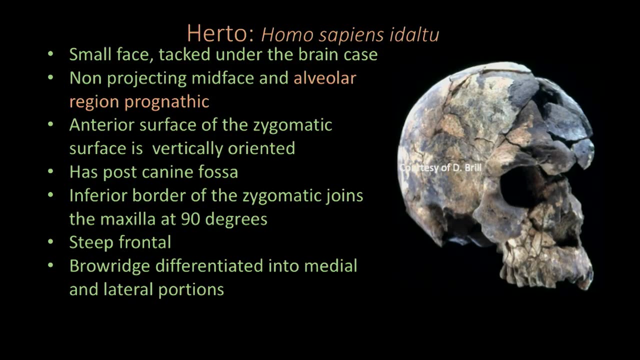 typical of Homo sapient. A steep frontal. that is major mark of Homo sapiens. steep frontal Brow ridge is differentiated into medial and lateral. The lateral part is thin and the medial part is thick. It's typical of Homo sapient. 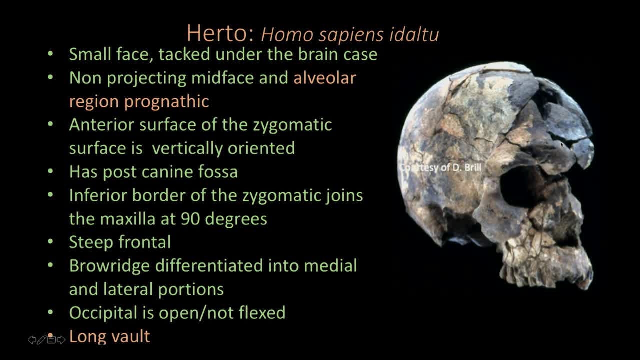 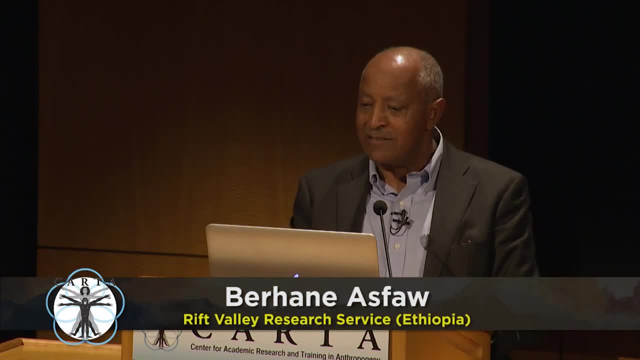 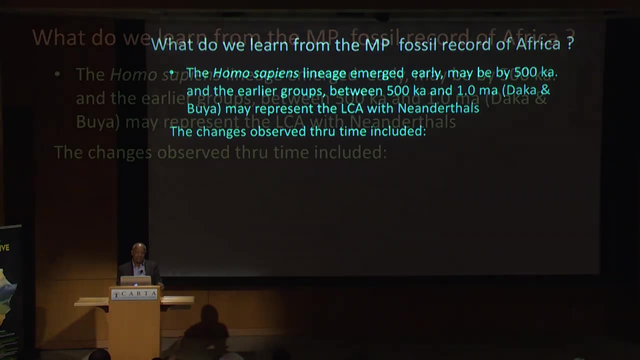 Occipital is open and flexed, Long, bold, but still has some primitive characters. So what do we learn from the middle plastidium fossil record in Africa? The Homo sapient lineage emerged early, maybe by 500,000 years ago. 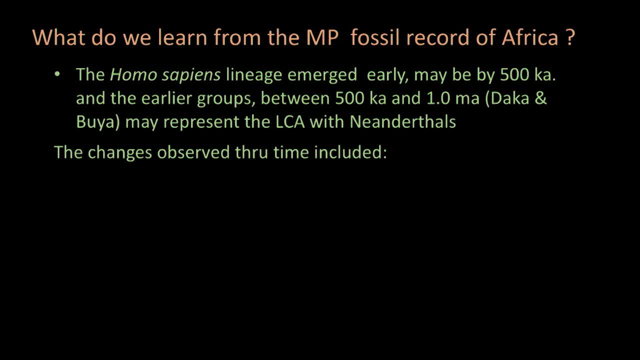 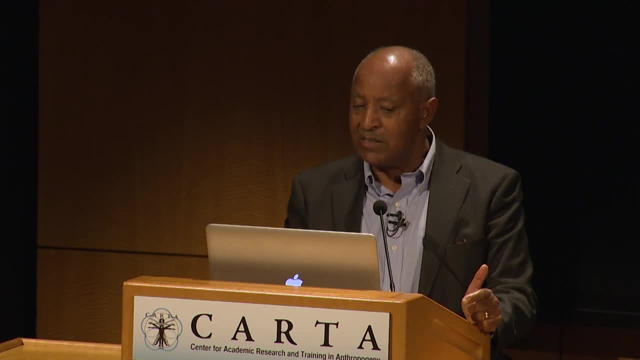 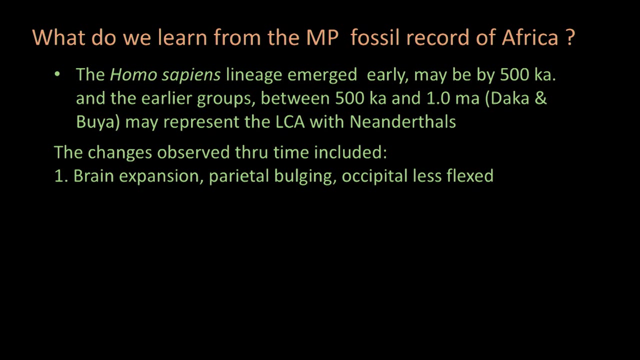 and earlier groups between 500,000 and one million years ago. Daka and Buya between those times may represent the last common ancestor with the Neanderthals. The change observed through time includes brain expansion that we have seen from Saldana time. 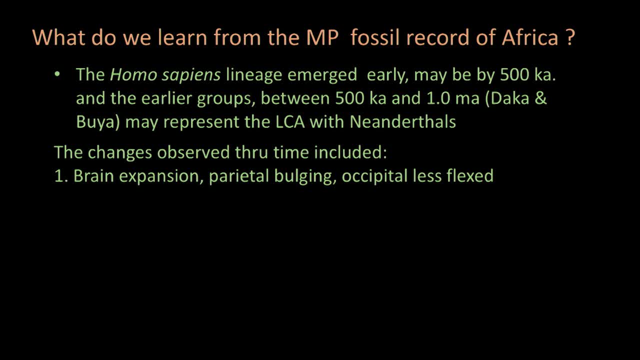 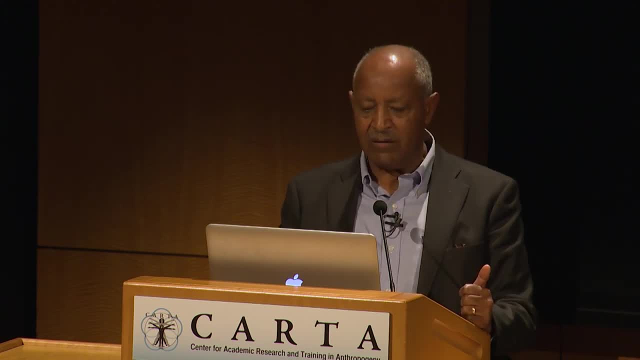 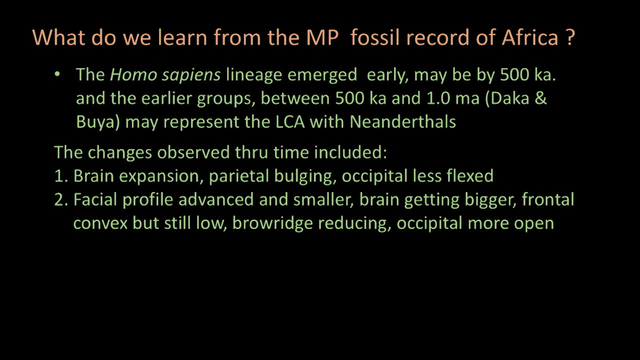 parietal bulging, as we observed also at Saldana time. occipital is flexed. that is that we have seen in, at least by Broken Hill. Facial profile advanced and small and smaller. that is what we see next by Ndutu time. 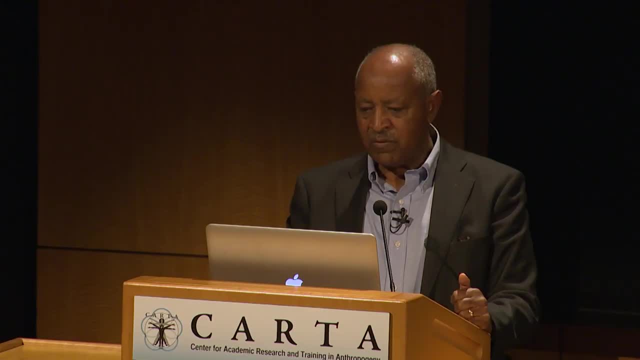 Brain getting bigger and frontal tips, frontal convex, but still low. that is what we see in Jebel Yohad Brow ridge reducing occipital, more open, Steep, frontal, smaller face. that is a third stage that we have seen. 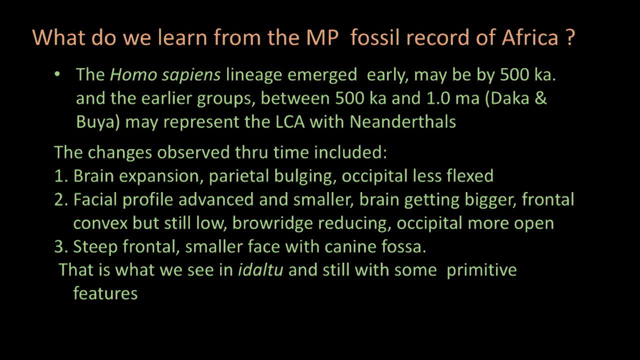 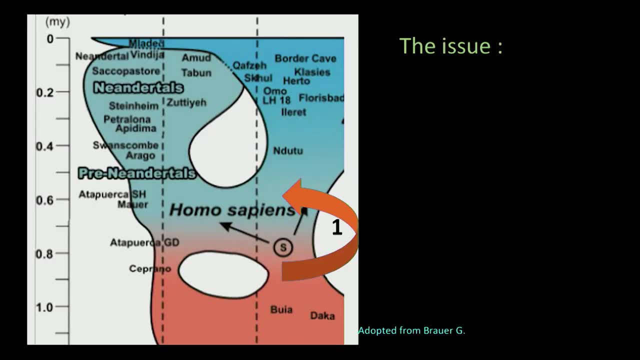 This is what we see in Idaftu, and still with some primitive features. Then, when we go the first stage, there is one stage, that's the brain expansion that we have started in the earlier parts, and the second stage.